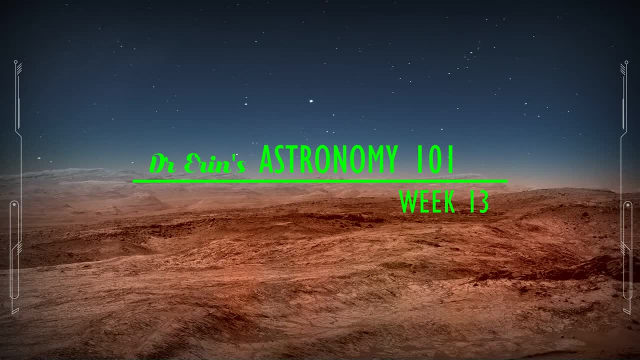 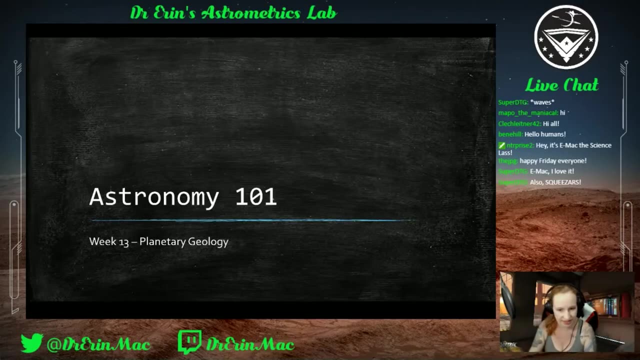 All right, so today we are going to be talking about planetary geology, mostly the beginning about this. We're going to go through kind of how the terrestrial planets in general formed, how they're shaped, the way they are, what's important about them, why the surfaces. 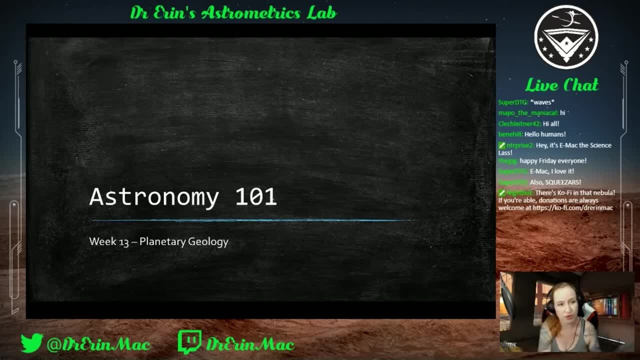 look the way they do. And then, if you haven't been here before, what we do is: this lecture takes about. this will probably be about half an hour, And then we'll kind of just do an AMA for the rest of the hour if we want to talk about any sort of random astronomy. 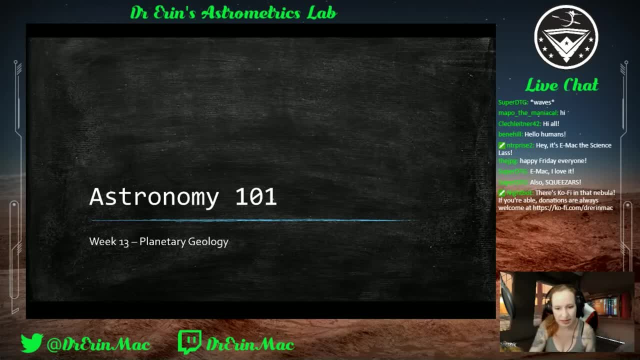 questions that we have or anything that's been happening lately, And if I don't know the answer, we'll look it up And I'll at least interpret the results for you, Because I have no shame in saying I don't know. But yeah, what we're going to do today is 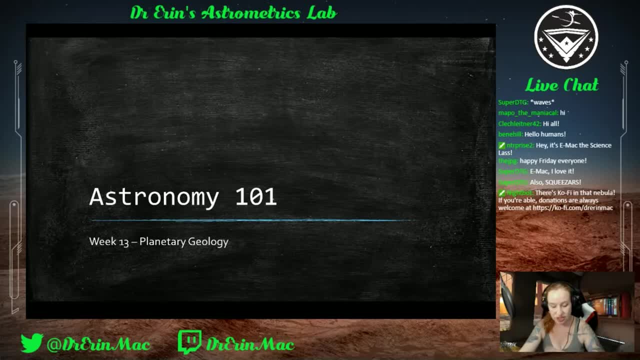 just kind of talk about the terrestrial planets in general And then we're going to just go through some of this planetary geology in general And then we'll talk about specific planets next week And if you're watching this live, you can stay here for the AMA. If 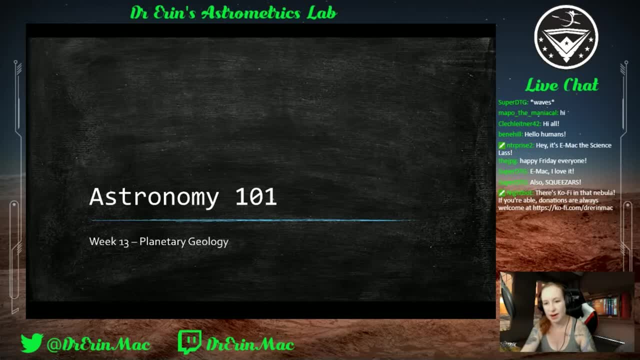 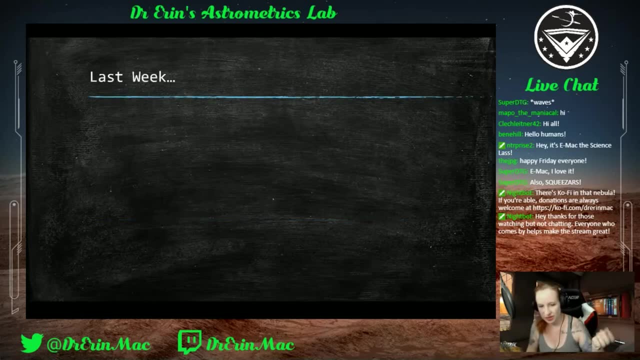 you are watching this after the fact on YouTube, then catch us live next time so you can take part. All right, So let's kick things off. So last week- not really last week, the week before, because I had to take a week off- we talked about the formation of the solar. 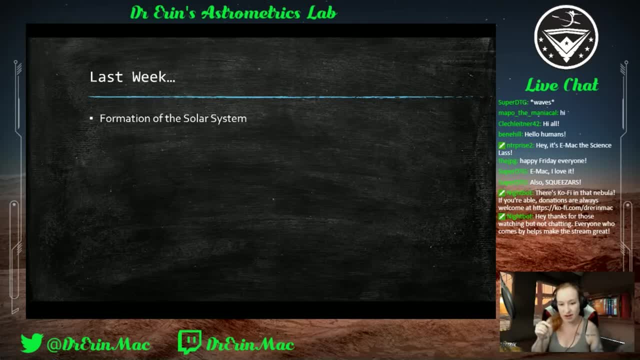 system And actually, if you follow me on Twitter, or yeah, if you follow me on Twitter, I'm going to talk about the formation of the solar system And I'm going to talk about- I just retweeted someone who had a great breakdown of this as well, But basically talking, 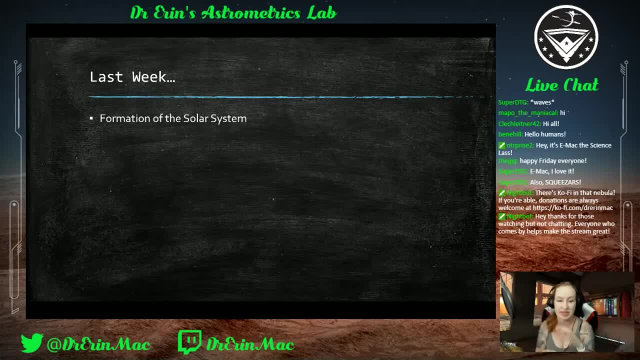 about how our solar system formed from a cloud of dust and gas And as it started to form we got these. you know these gravitational impacts that that are happening. you start to get these little dust particles, that kind of coalesce, run into each other, get a little. 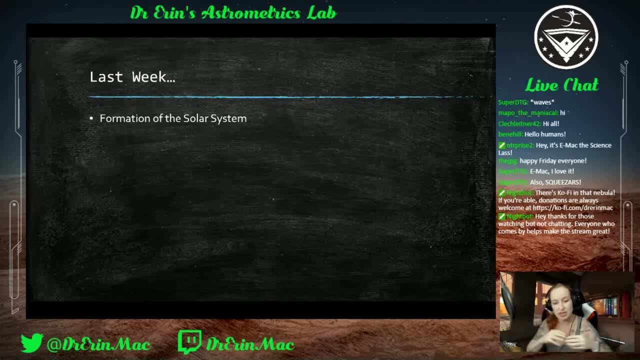 bit bigger, increase their gravity, so more stuff crashes into them and you get this like snowball effect And in the middle you get this really sort of hot. it starts to heat up because of friction And it starts to get really dense And then, once that has reached this sort of critical, 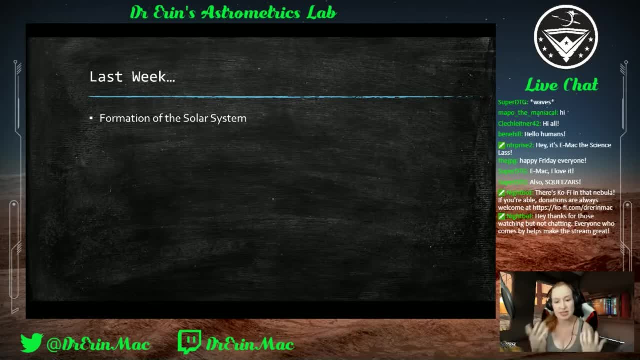 temperature density, it starts fusing the hydrogen gas into helium And then at that point we have a star. However, as that's been going on, all of that dust and gas has started to kind of coalesce and shrink down through gravity and angular momentum. and these 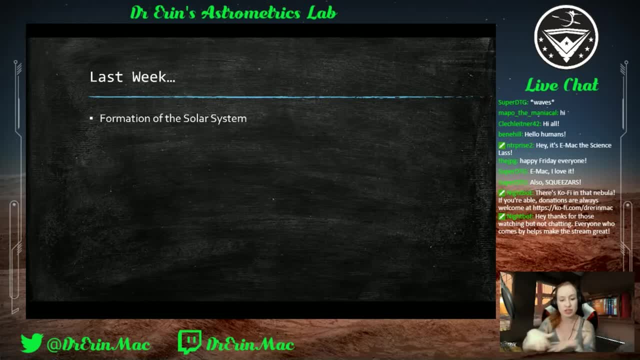 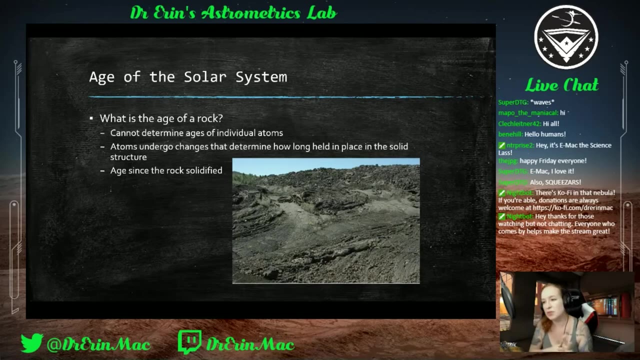 random processes, that averages out to be a flat disk. And then we get these planetesimals and those planetesimals start to clear out their orbit And- and we'll go through today how we get these terrestrial planets. So when we talk about the age of our solar system, 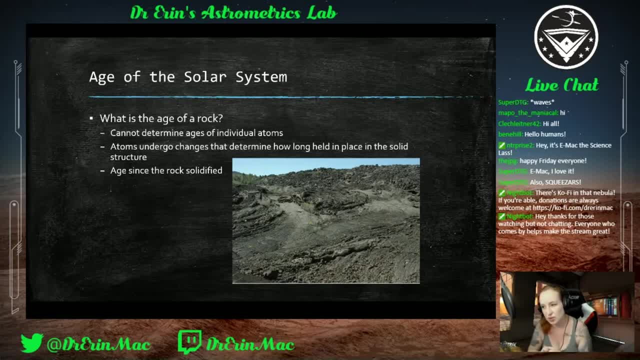 remember we're saying that our solar system is about 4 billion years old. One of the things we can do is try to determine, through the age of rocks Now, if we're pulling out an individual atom, whether that's hydrogen, carbon nitrogen, anything you can't just. 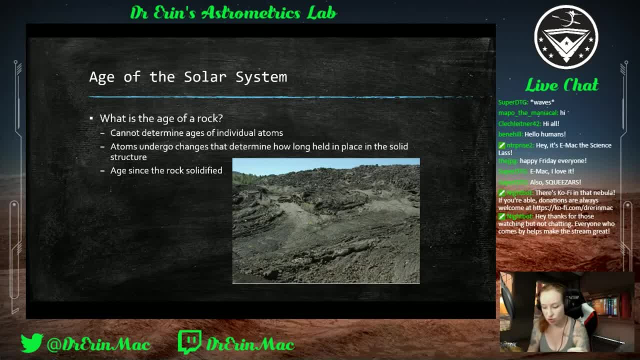 look at a single atom And determine how long it's been around, how long it formed, However, that if you have a solid structure that's made up of atoms, then those will start to undergo changes that determine how long it's been held in place in that solid structure. So what we're really. 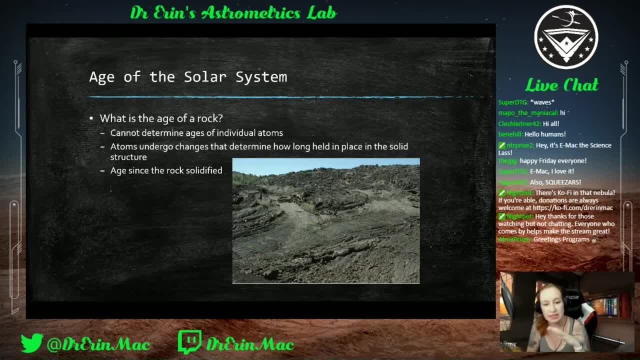 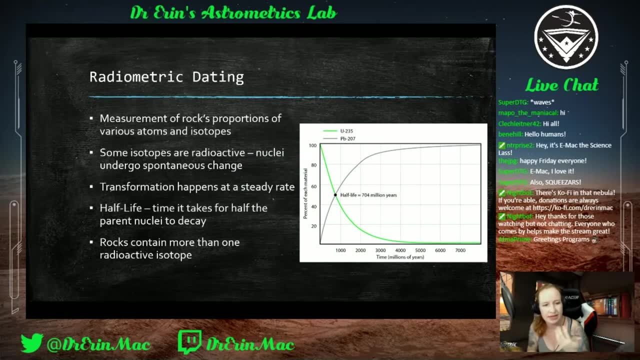 doing is we're finding the age since the rock has solidified. Hey Atma, How we go through this is actually called radiometric dating, And we talked about this a little bit, I think, actually in our talk In our episode club, when we were talking about how in the Star Trek Next Generation. 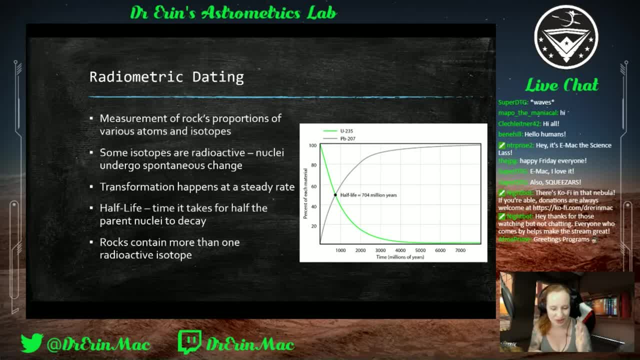 All Good Things. they could tell the proportion of air molecules that were in Picard's lungs to determine that he hadn't been off of the ship, And then figuring out how much time had passed based on that. So it was pretty, pretty intense. Hey Trek nerd, I'm glad. 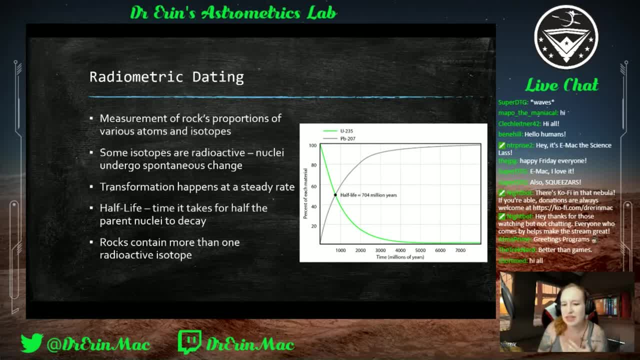 So this radiometric dating, basically what we're doing is we're measuring the, the rock's proportions of different atoms, We're measuring the different atoms and isotopes. what we have, So remember, isotopes are, when you take an atom, atoms are made up of protons and neutrons and then they're orbited by. 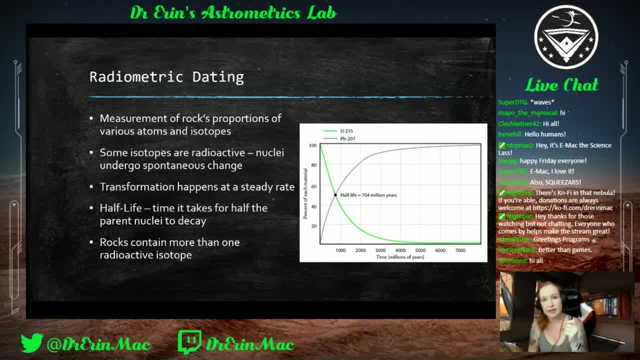 electrons. The amount of protons that are in the atom determine what element it is. So you know, two protons is a helium atom, And then we have six protons. That's usually the best one. Six protons is a carbon atom. Hey, short man, And typically you'll have an atom. 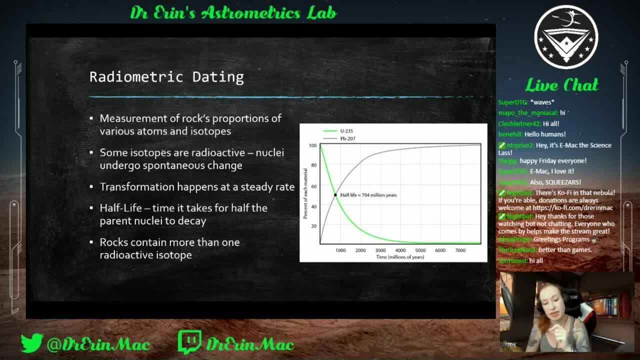 an equal amount of protons and neutrons, but sometimes the amount of neutrons can change. So if you've heard the term carbon-14, what that means is you have six protons and eight neutrons, And those are what we call isotopes. So if you can measure the proportions of different 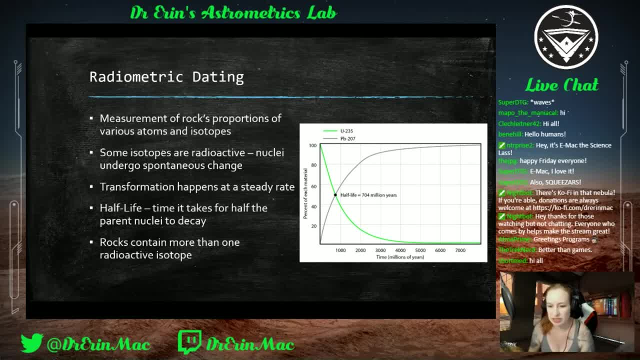 isotopes that can help us do radiometric dating, And the reason that it's good for this is because some isotopes are radioactive, And when we say something is radioactive, what we're really saying is that that nucleus, that the protons and neutrons they're going. 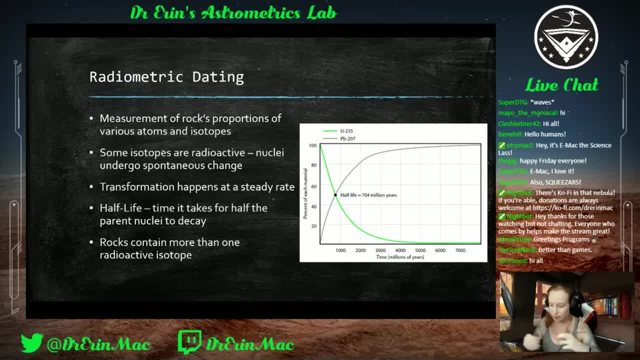 to undergo spontaneous change. They'll spit out protons or neutrons, and then they'll. they'll change themselves, And this transformation that happens overall, happens at a steady rate, And so the way that we measure this is something called the half-life. So you have this, you. 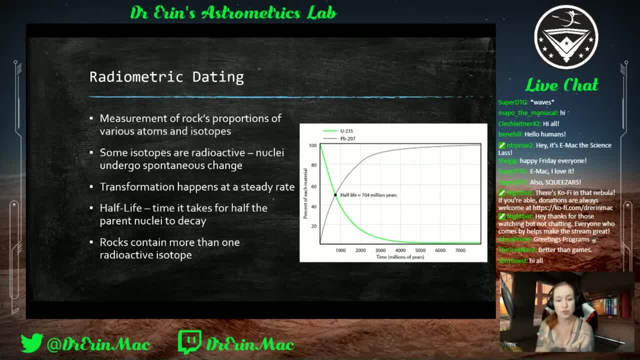 know set of isotopes and those isotopes, over time, are going to go through these random changes. Um, but that random change when you're talking about, you know thousands are here. I don't remember things like a mole's worth Avogadro's number, anything like that, Um. 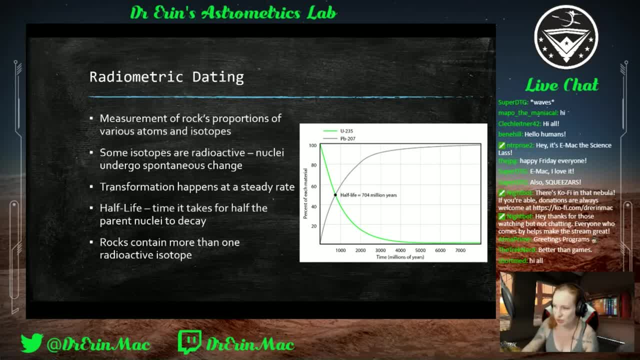 overall, that will follow a steady process, which is what you see here. And then we determine: the half-life is the time it takes for half of that parent nuclei, that that isotope that you're starting with, to decay. So it's half of it has disappeared and it's changed. 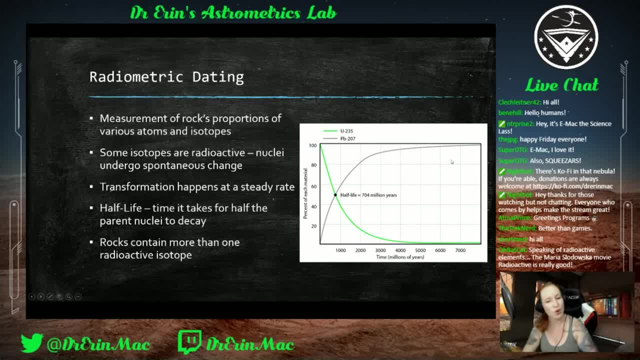 into something else. Um, Hey, Becca. Oh, good to know. Thank you for the recommendation. Uh, so uranium-235, that's basically saying it's um weight- is uh 235.. And remember, that's the combination of protons and neutrons. 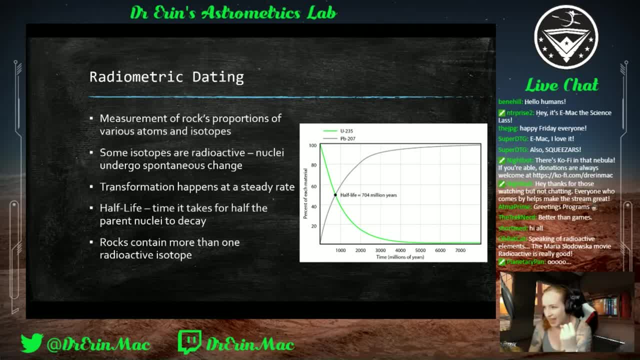 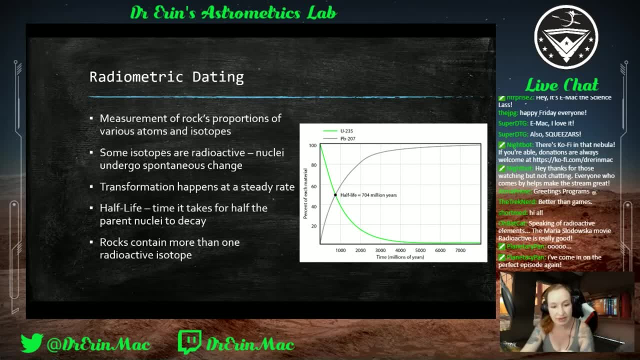 that are in there, Um, Hey, Planetary. And what that does, is it actually? um, it decays and then that's half-life of uranium-235 is 704 years, Yay, Um, and these rocks, uh, can contain more than one radioactive isotope. So that's really helpful, because sometimes 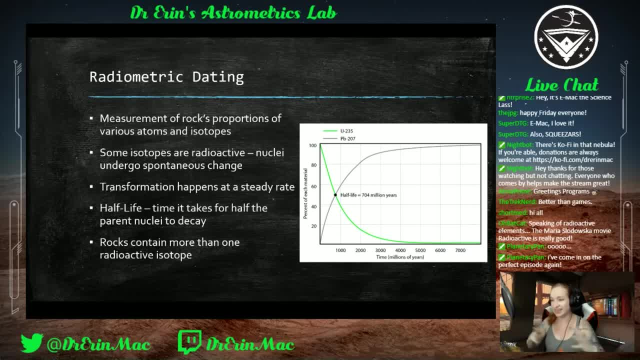 it might not be. you know a whole lot of material You're not getting. you know cause you want to get this average. you want it to average out so you're able to get a good read on how old it is, but rocks will contain more than. 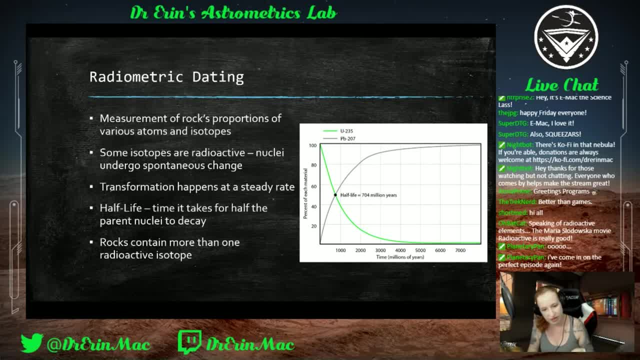 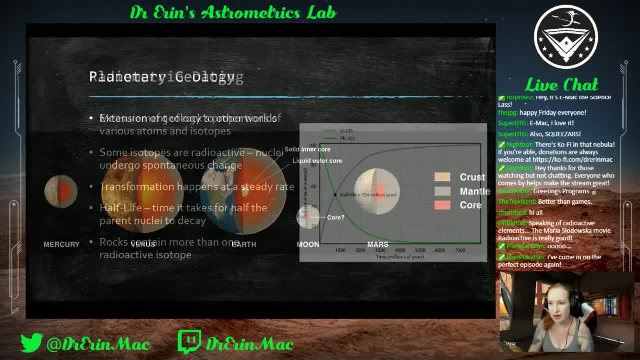 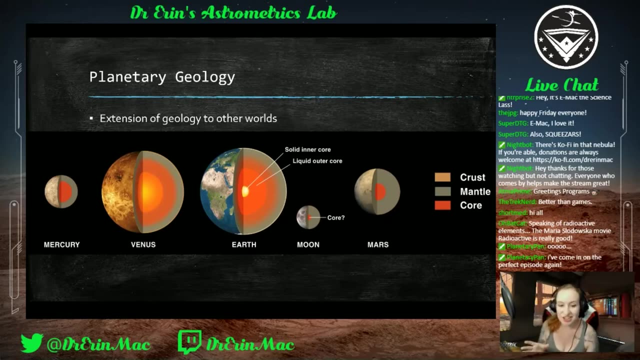 one radioactive isotope So you can compare them all. knowing the half-life of these individual isotopes can help you determine, um kind of, what your your baseline start was and how old the rock is. Now, when we talk about planetary geology, the term planetary geology 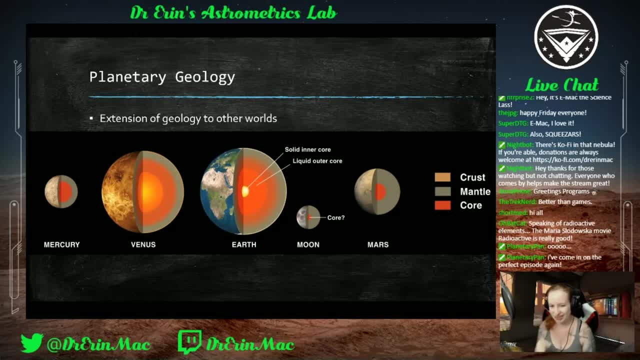 geology. officially, geo means earth, the study of earth. So when we say planetary geology, it's kind of like an AT. it's not even an ATM machine, It's the opposite of that. uh, that it's exactly not of what you're talking about, but um, 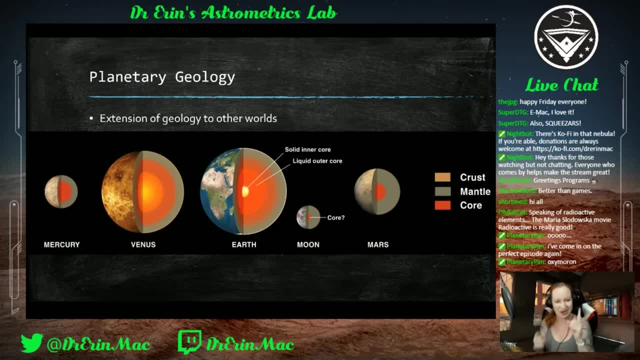 it's just the extension of geology to other worlds. Yeah, Oxymoron, That's the correct one. Thank you, Um, so, because we remember, our solar system is broken down into four terrestrial planets and four jovial planets- jovial, it's been a week- Jovian planets. 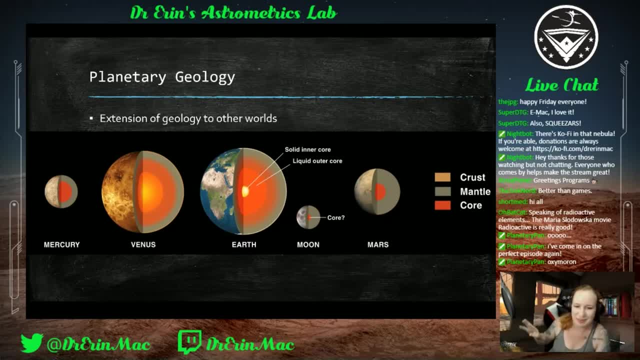 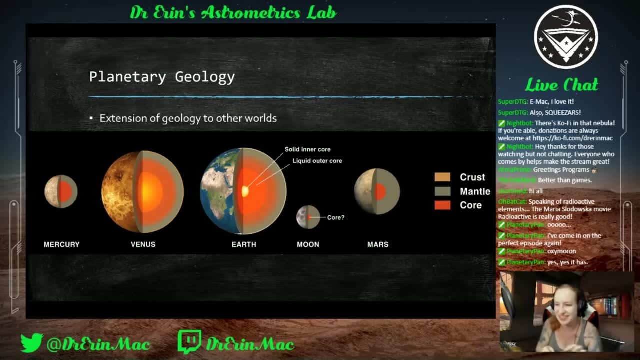 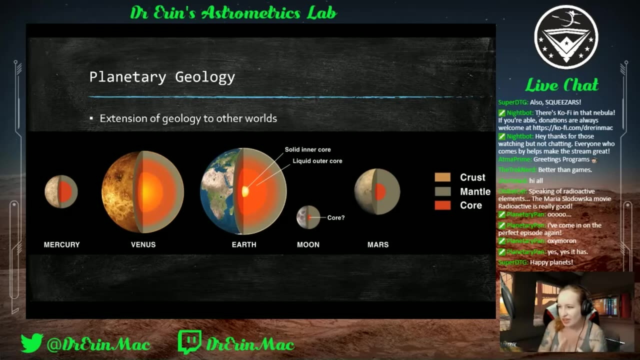 Okay, Okay, Jovian planets- I suppose they're happy Jovian planets- And then we have our- uh, we have our dwarf planets, our asteroids, all of those other things, Um, but if we're talking about our terrestrial worlds, um, we have Mercury, Venus, earth and Mars, and then we kind of 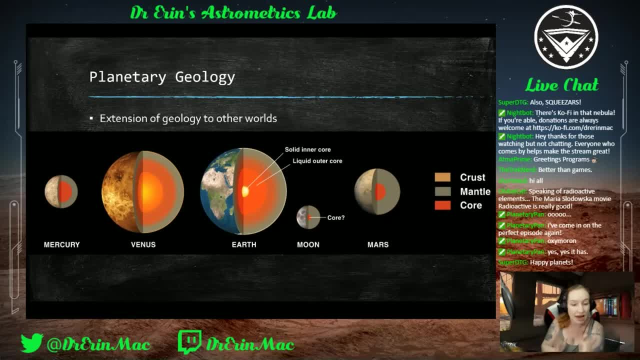 throw the moon in there too, just because, remember, the moon is one of these outliers in finding patterns in our solar system. for the terrestrial planets, It's incredibly large. It's a large moon in proportion to the other, Uh to to its parent planet, us. um, Mars also has moons, but they're like small potato. 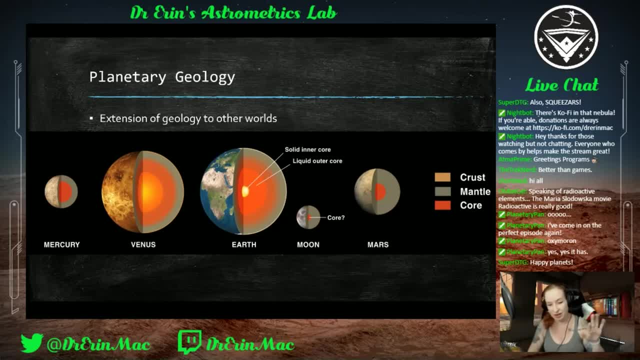 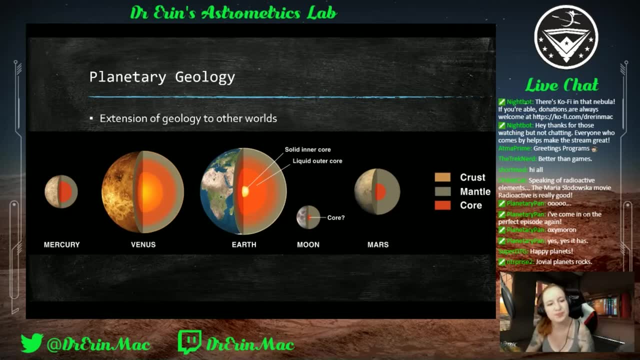 shaped moons. So, uh, the moon is an outlier. We can kind of call it a planetoid planet, like and um, yeah, and we can study that as well. So what we've been able to learn through various studies, whether we're doing sort of um radar studies, uh, or measuring- 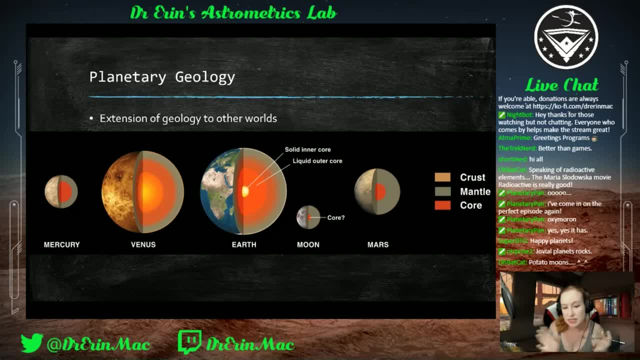 sort of the magnetic field or building computer models to see how we can get this, this stuff out. Yeah, Um, we can start to build up what's on the inside of this. So we have these three major components that are the crust, the mantle and the core. And if you remember from school, 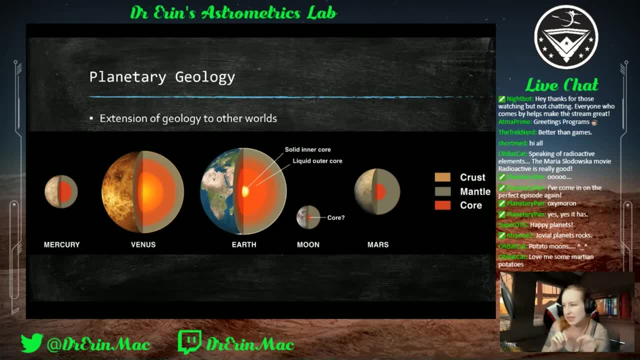 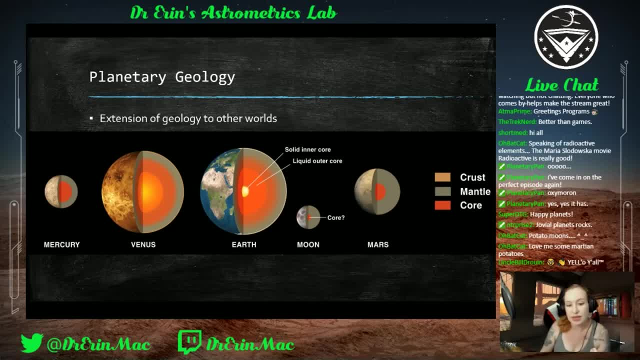 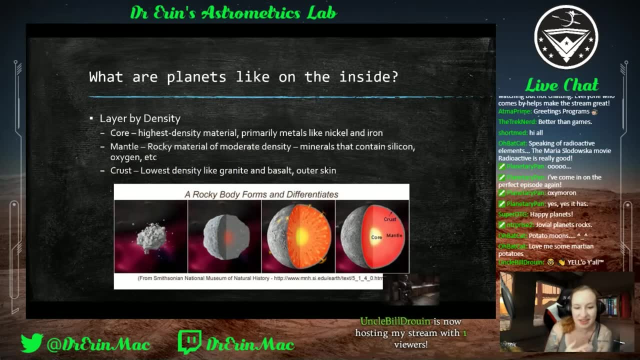 Particularly with Mars. that changes how we can determine what type of interior it is. Hi, Uncle Bill. Alright, so what planets are like on the inside? it really layers out by density. Oh, and, thank you for the host. All right, this core, like I said, that's the highest density material, That's in the middle, That's in the core. 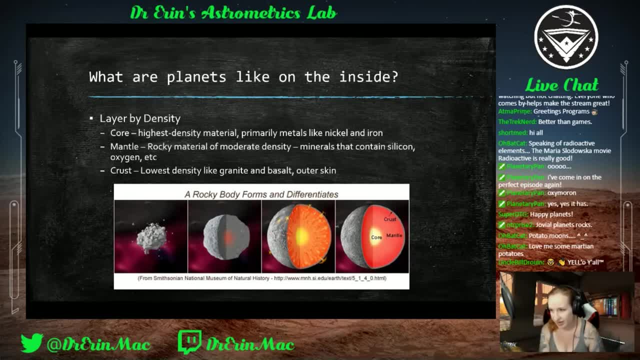 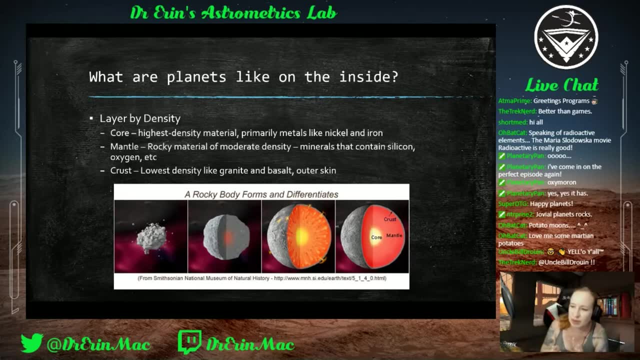 It's primarily made up of metals like nickel and iron, Then outside of that, the majority of a planet. here We have the mantle. now this is the rocky material. It's moderate density and it's gonna be more minerals that are like silicon or oxygen, and that's gonna be a big part of that too. 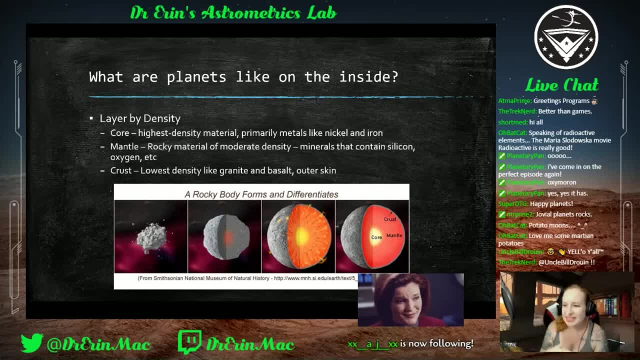 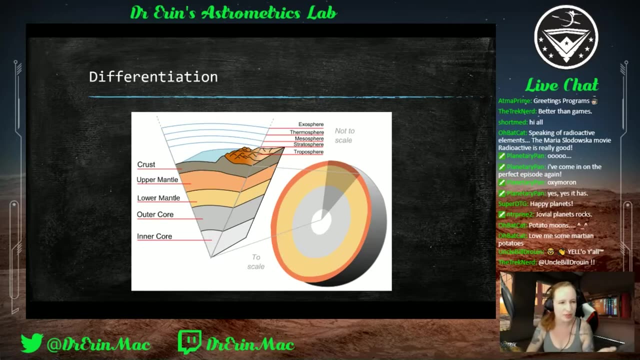 Oh, thank you for the follow. And then, like I said, the crust is this really thin outer skin and it's the lowest density, like made up of granite and basalt, And how this sort of shakes out. It's really important to note and it's one of these things that maybe, if you haven't thought about this, you're realizing it for the first. 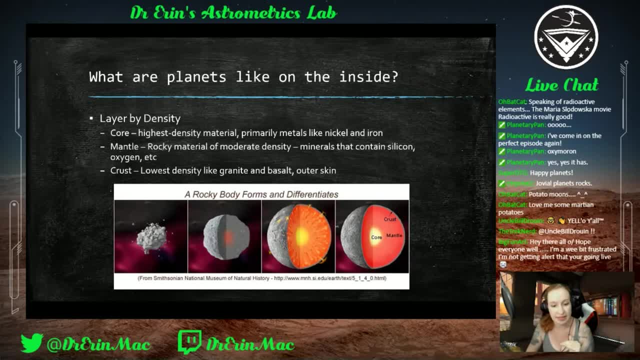 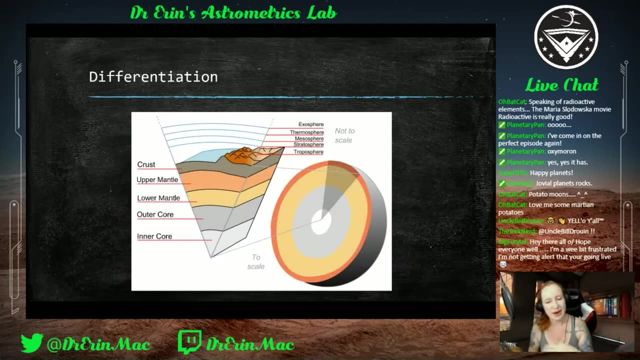 Time and that's okay too. But remember, I'm saying layering by density and the way things, the way things that can Differentiate- I'm trying to use the word without actually saying differentiate. the way things separate by density is called differentiation. I'm sorry to hear that big fun art. 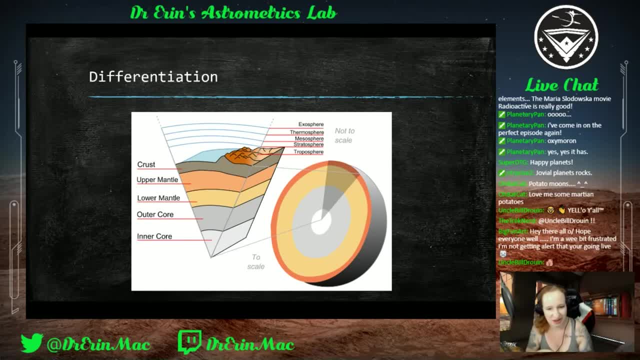 I will dig into that a little bit to see if I can help with that at all. It may be something I might end. there's still some nuances that I that I try to figure out, but I've definitely heard that before. I also have a discord channel, but that that you. 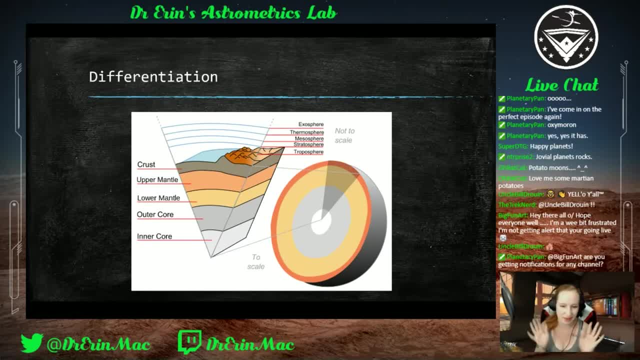 usually takes about five to 10 minutes for that notification to go up. Anyway, Um, all right, So differentiation, that's where you, I mean, think about it this way: If you've played with the oil and water, right, You shake up oil and water, or vinegar and oil. If you're making salad dressing, 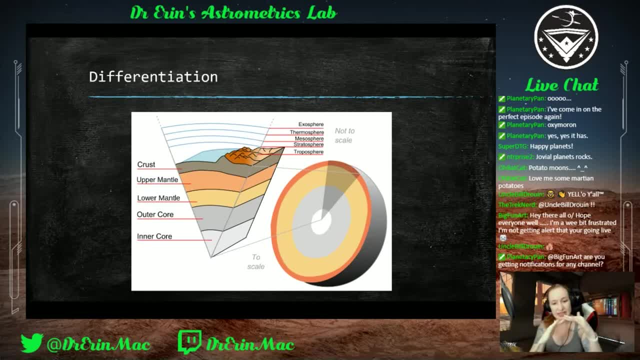 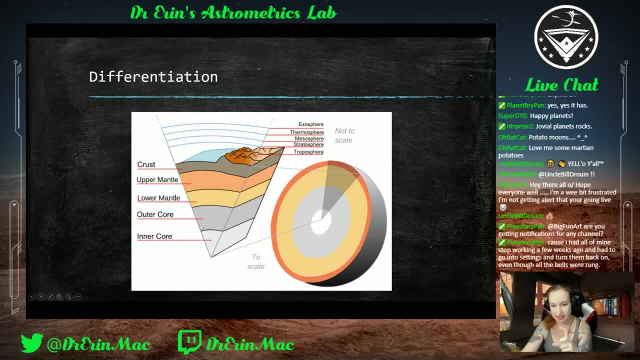 something like that. If you shake it up and then let it sit, what it's happening is it's differentiating, and it's basically separating by density, And so that's how we end up with this: the core, the highest density, then the mantle medium density and then the crust is the thin. 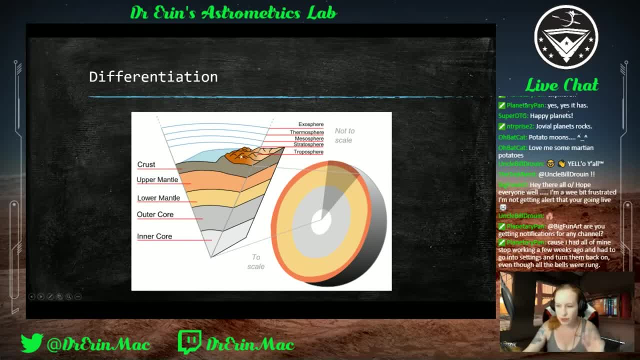 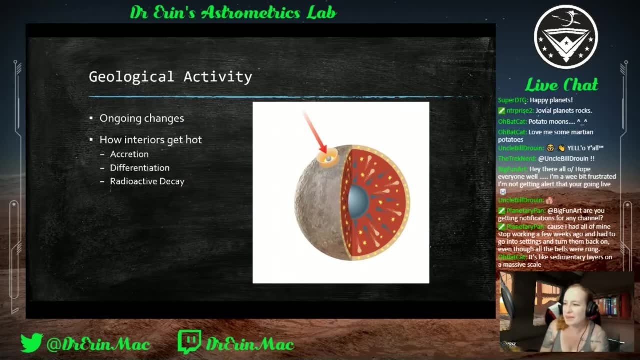 layer And um, and then we also have differentiation in the atmosphere as well- Note that it's not to scale- And um, all of that that differentiation as a planet is forming actually dictates how the interior layers of a planet get hot. And yeah, Becca, that's a really. 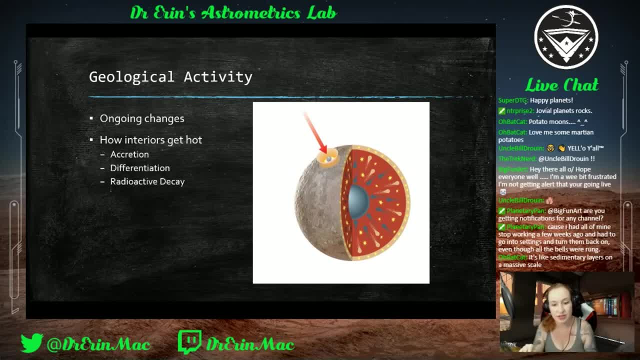 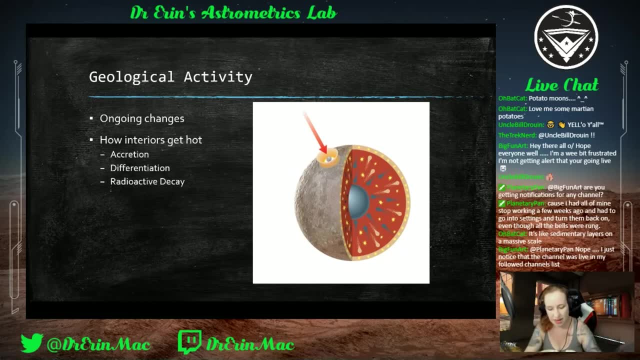 good point too, that when you're talking about sedimentary rocks and the layers there, that's essentially what's going on, because sedimentary rock, that's the layered rock, And then it's just um, and then what it's doing is: 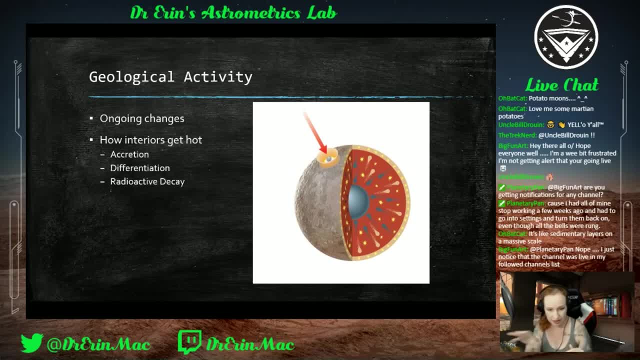 it's settling out the heavier material, the rocks, in this liquid- So typically a lake or an ocean or something- the the rock layers will settle down and then the geological processes happen, More rocks are introduced and then they layer down again, And so you get these layers of rock as 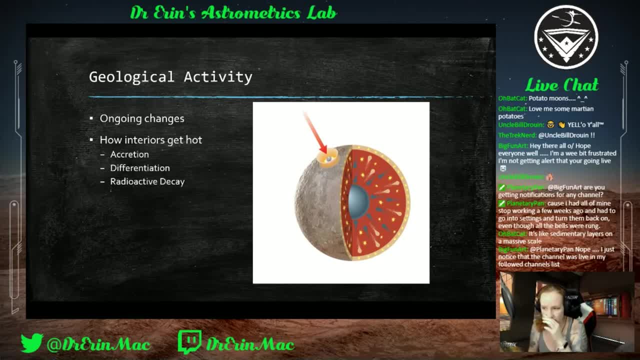 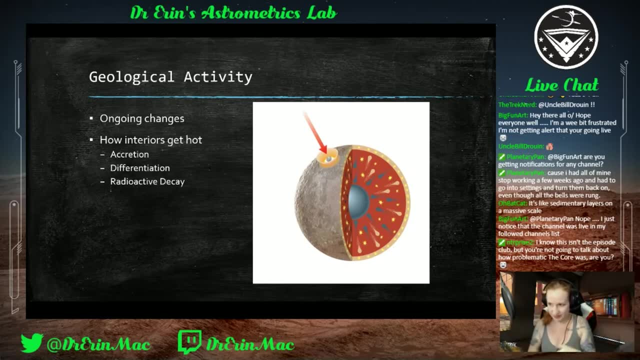 you go and that's how you get sedimentary rock, And we're going to talk about that a little bit here as well. But the ongoing changes that are inside of a um of a planet include uh, accretion, differentiation and. 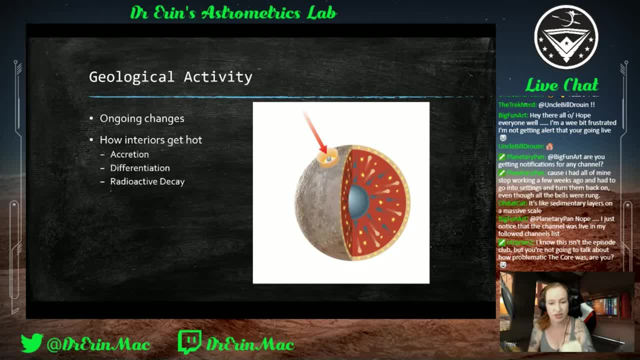 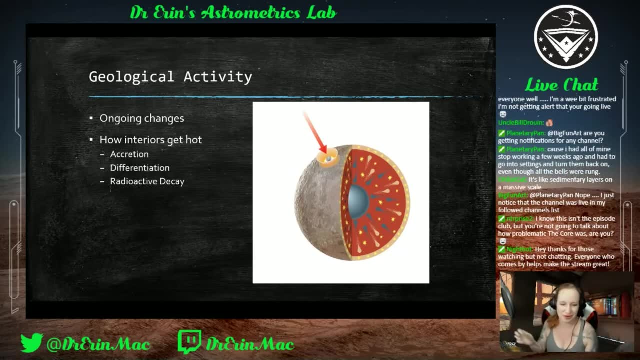 radioactive decay all contribute to a hot interior on a planet. Billy, All I saw was episode club in the core and wondering if, like yeah, people were like, yeah, that's um. so the core. Let's save that for the AMA at the end. 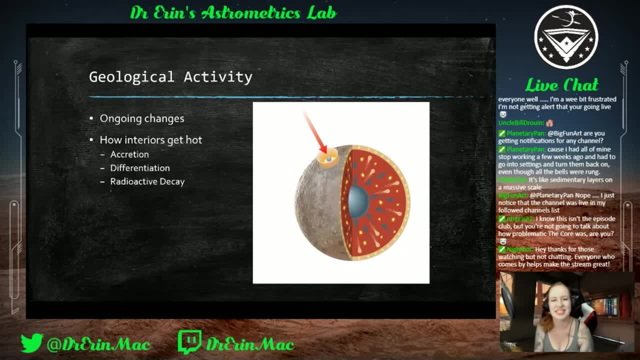 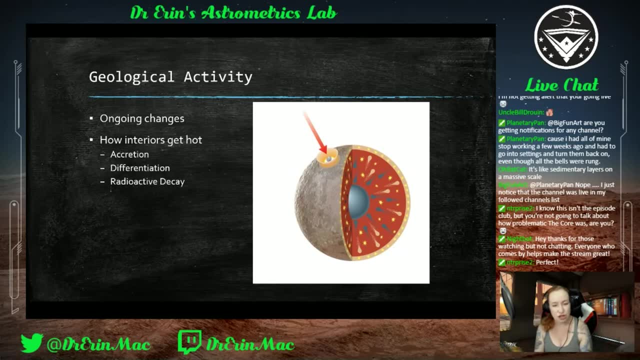 Where we can talk about, because I I'm going to need, I'm going to need some reminding. It's basically the core stopped and then they tried to bury a nuke right To restart the core. Yeah, We'll talk about that at the end, but be prepared to remind me exactly what the plot was, because 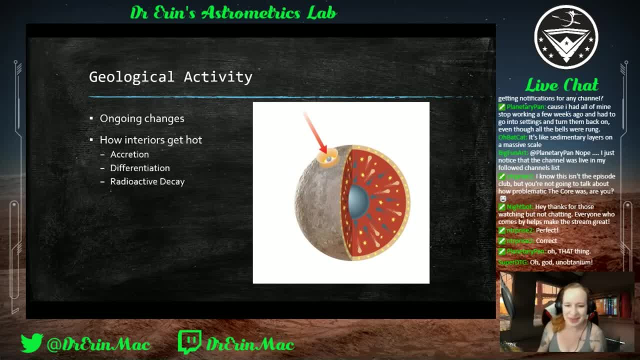 it's been a long time and that movie stressed me out: Um, yeah, Okay, So, uh, accretion, that's kind of what's being demonstrated here. We have stuff that's crashing into the planet, So it's, it's building up the planet. But remember when we learned about energy, conservation of energy. 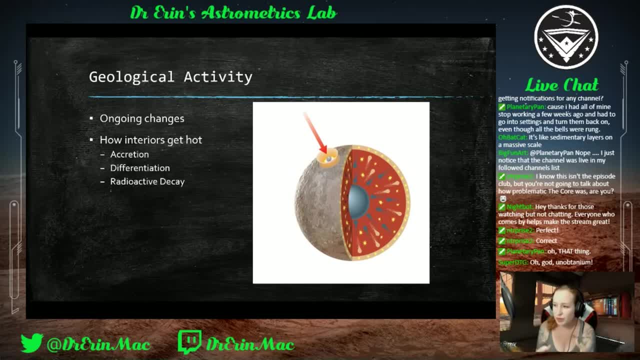 um, and trans energy transfer. what we have is, when something crashes into a planet, uh, that is coming in and it has kinetic energy, because it has a speed and that. and once it crashes, though, that kinetic energy has to go somewhere, And now that can be transferred, because we have kind of a 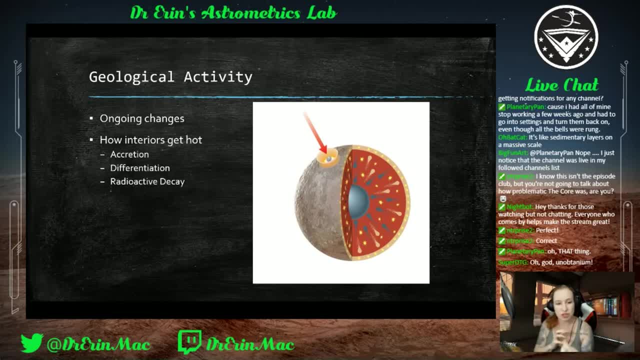 collision that's happening. So if it's really big, you can think of a transfer of momentum, So that mass and the velocity is now, um, you know, a, uh, a non-elastic collision, that it's gone and it's attached, Um, but also you can lose energy from thermal energy. So when it crashes, 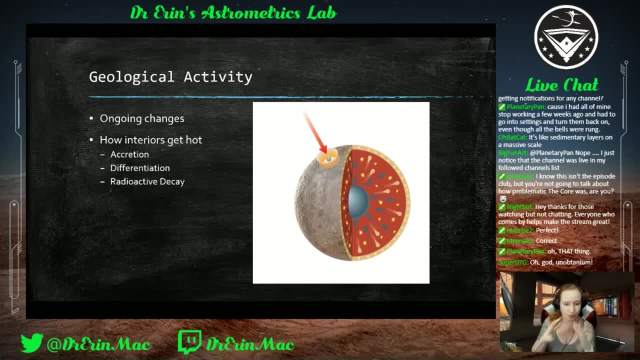 it's going to transfer some of that energy to heat. That heat is going to contribute to um a hot interior. And this is particularly important when we're talking about the early formation of planets because, remember, there's that whole period where, um, it's all kind of shaking out. 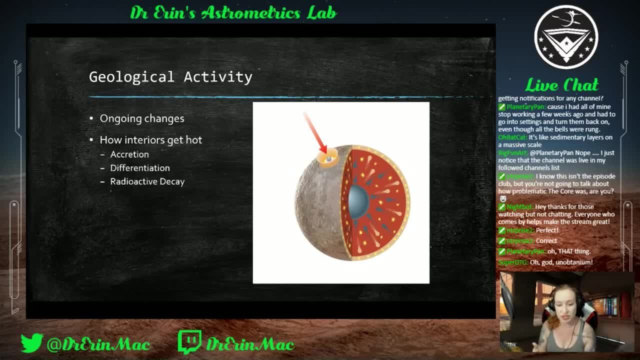 of chaotic processes are happening, Lots of things are running into each other, And even as these planetoids are starting to clear out their orbit, they're still running into a lot of stuff. So it's this accretion That's what's going to be building up a lot of heat on the planet itself. 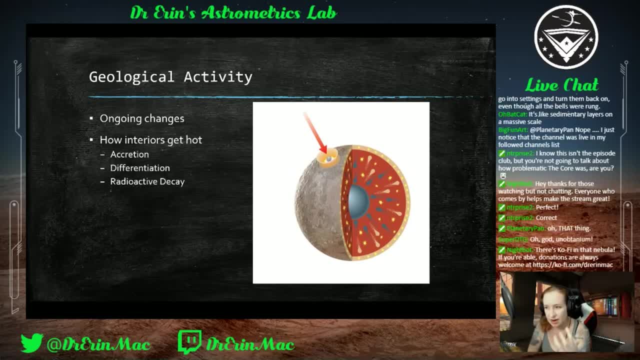 Differentiation is going to be a major part of this um heating of the interior. So again, when you think about the early formation of a planet, we just have a lot of hot crap. It's all kind of coalesced with itself and it's all starting to um come together. Oh, thank you. 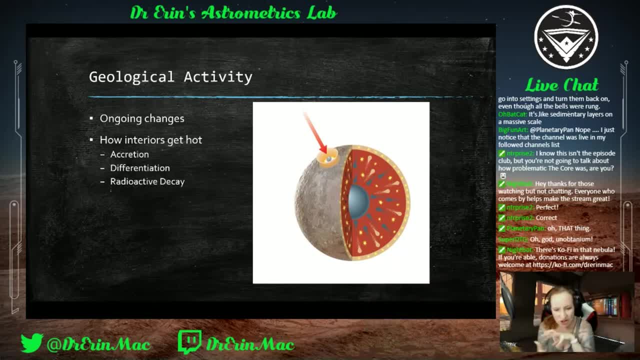 Lake girl: Yay, Um, it's all kind of come together, but it hasn't settled out yet. So we have different minerals. Remember when I was talking about how the mantle and the core and the crust are all made up of different um, minerals, atoms, all of those things. those are all just mixed together. 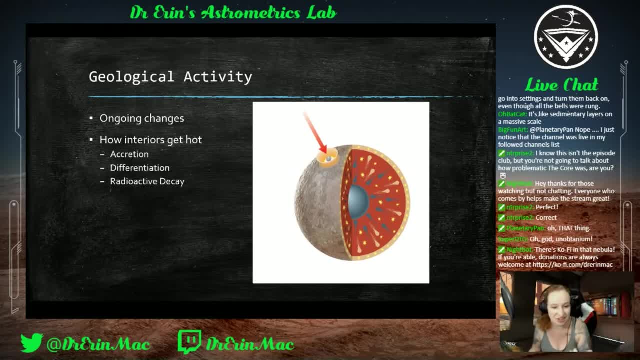 And one big thing: this is like when you've just shaken up your salad dressing right, Then you let it sit, that sitting process. Once it's cleared out its orbit, it's got a lot of accretion, It's kind of built itself up. Then that differentiation is starting to take place. 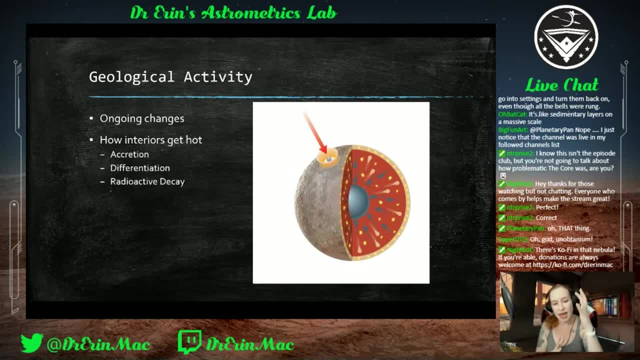 And so now we're starting to get things to settle out And as it's transferring- where you can see here this hot, you know- the heavy gray stuff is going to the middle, The lighter stuff is moving to the outside. as it's moving, we're having friction. you know that that's going on. 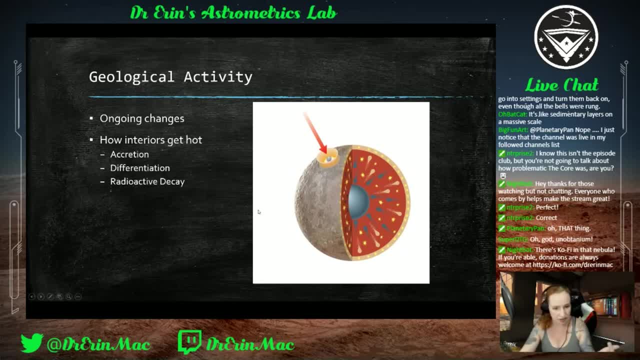 And so that's contributing to some heat as well. And then the material themselves, uh is uh undergoing radioactive decay just because they'll, they'll be made up of unstable isotopes, And some of them have been incredibly long half-lives. Uh, so the idea that you could 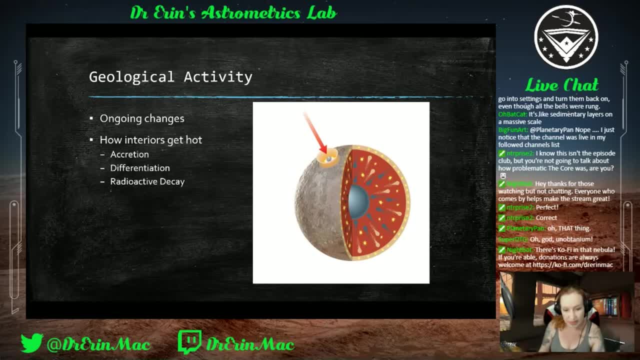 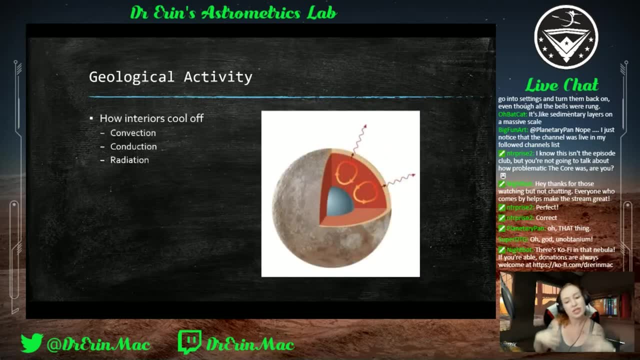 have uranium 235,, for example, be a part of this and undergoing decay. that contributes to the heat as well, because when it decays, it gives off some energy. Okay, So now we have our planet. we have a hot interior, we have a crust, it's all kind of settled out. We have our layers. 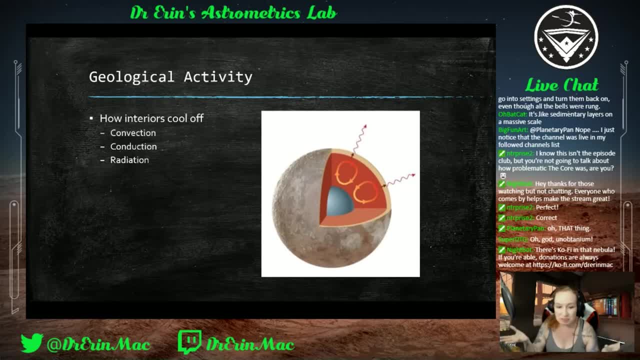 we have our core, our mantle and our crust, Then it's basically going to start cooling off. And how that cools off is once these layers have all kind of settled out, we get this convection, conduction and radiation, And I want to make sure I say this right. 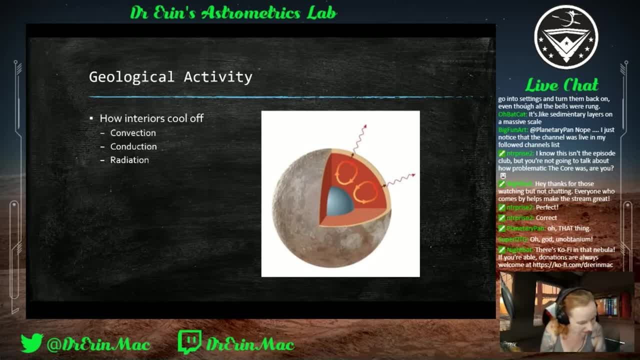 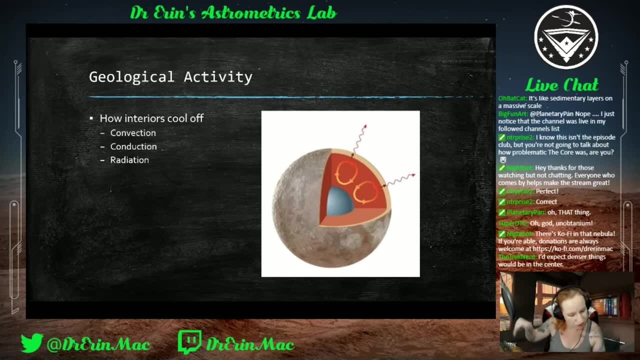 because I never say it right And I'm okay with that. Um, so convection is where you get the hot material expanding and rising up and then cooler and then cooling off and following back down. So it's bringing heat up and then it loses that heat and it goes back down Convention ovens. 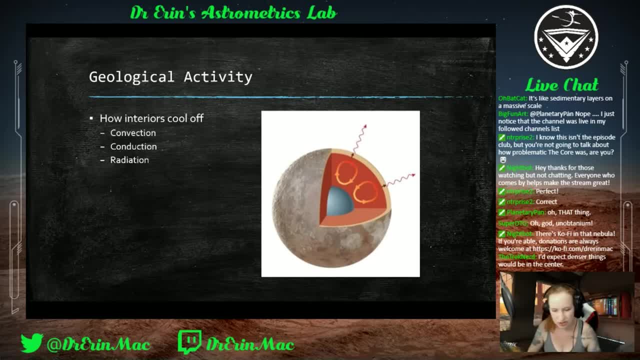 Yes, The denser things are in the center. Did I say that? backwards Trek, nerd. Thank you for catching that. It should be. That's what it should be. Um, if I didn't say that, then that was wrong. 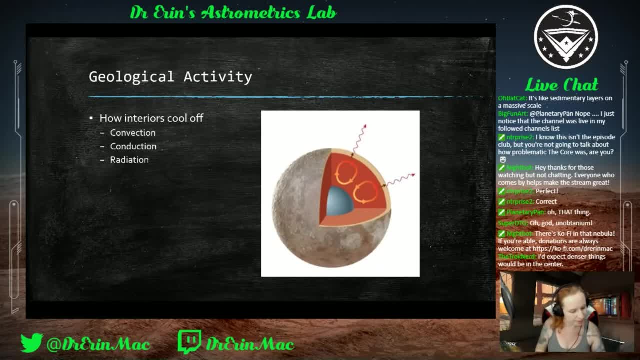 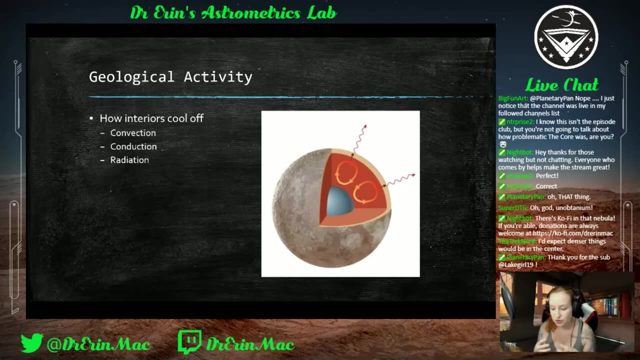 Um, so I apologize for that, but thank you for catching that. Um, and then conduction. Okay, So convection, think about convection ovens. right, The hot air rises, cools, falls again, And then that's the uh convection process And that cools off, um, because there's little, it's not totally. 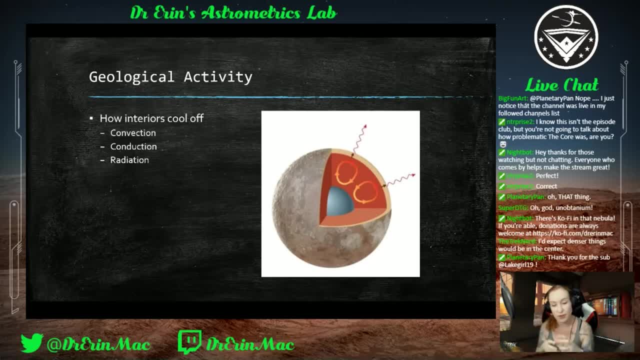 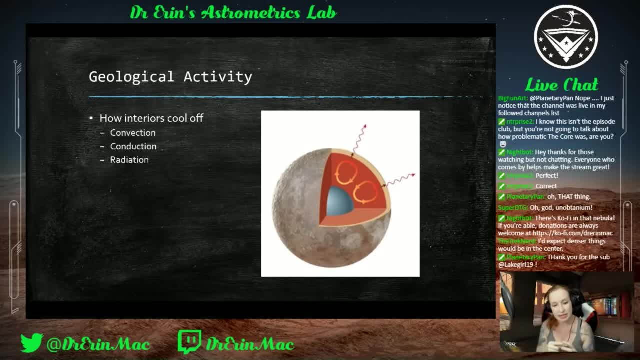 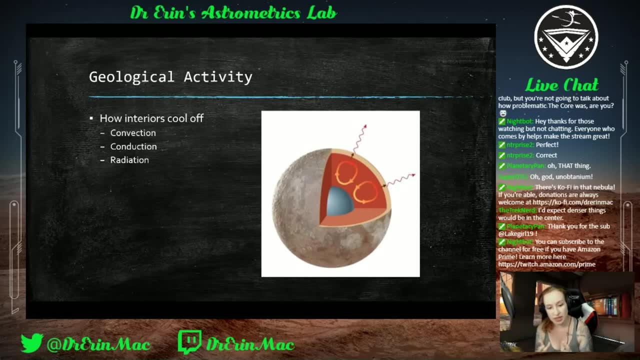 it starts to cool off and then it falls back down again And then it's still heats up because the hot is still, the center is still warmer. So it heats up and it rises again And then conduction is that process of, as that material is rising, it's cooling off because it's hot and it's meeting. 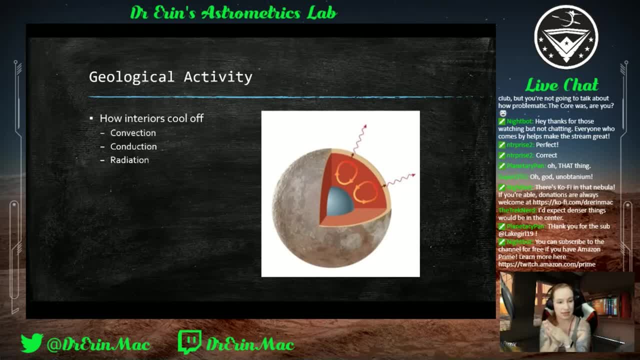 colder things And there's a heat transfer process. that happens. That's um conduction, And then radiation: is the heat actually leaving the planet itself? That's where it's radiating off. It's um. you know where we talked about that black body radiation, the thermal curve that we 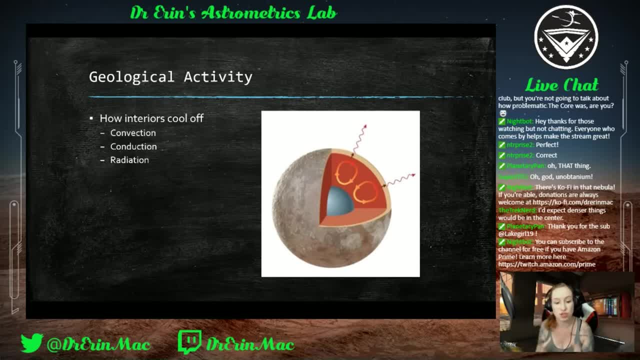 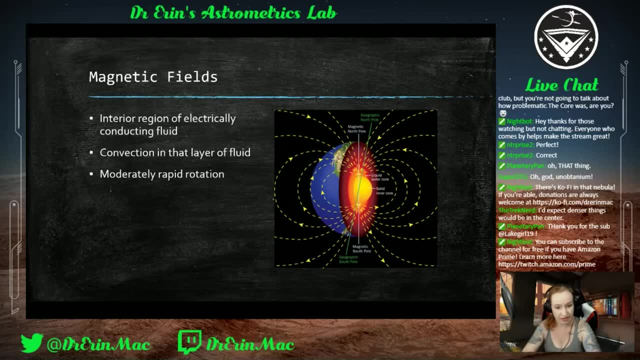 get. Um, that's how all of these processes start to slowly cool off the planet. Okay, Then we talk a little bit about the magnetic fields, and this is kind of where the core comes into play. here, but the uh, we have this interior region and it's going to be high metals, right, Because this is 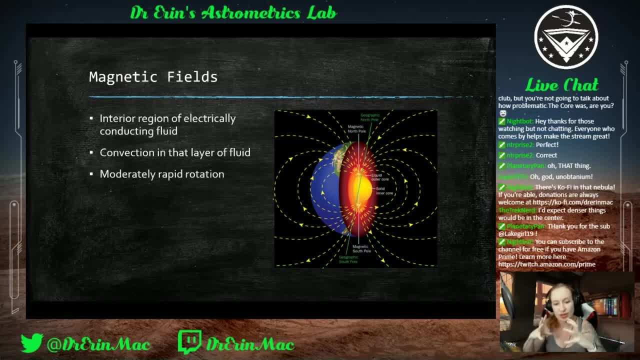 the most dense is going to be at the center And then we have that inner core, the outer core, we have the inner mantle and the outer mantle and we're going down in temperature as we're going out. we're going least density as we're going out, but near that center part, particularly if we have 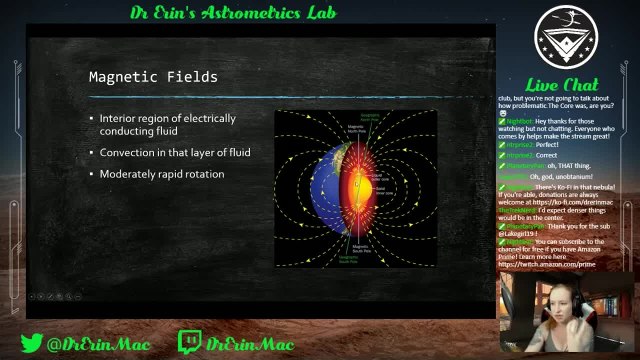 this outer core. that's liquid that's going to be rotating and the convection that's going on. So we have electrically conductive conducting fluid. We essentially have metals here that are able to conduct electricity. We have convection that's going on where the heat's rising and then it's falling again. all in this, 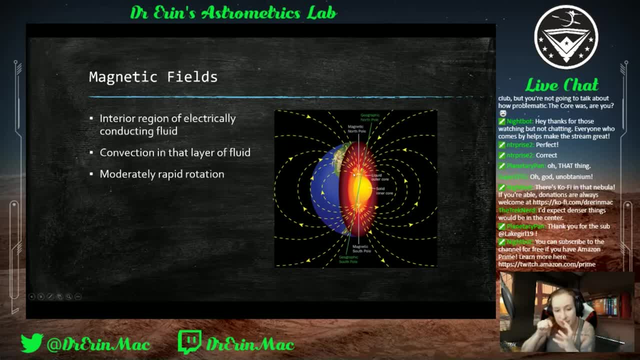 uh, this core here, this liquid outer core, because it's going through that process, is basically generating an electric, electromagnetic field that then propagates through because there's kind of nothing to stop that. That's where um, the core itself, the fact that it's metal. 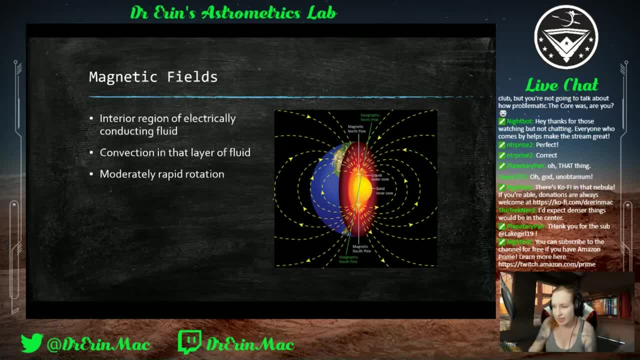 that's the magnetic part That creates this magnetic fields throughout the planet. So I hope that makes sense. I know I kind of burned, burned through that a little bit. Um, let me just make sure I didn't miss any, any of the main points here. Um, so in, or I guess it's important to note that if you don't have this, 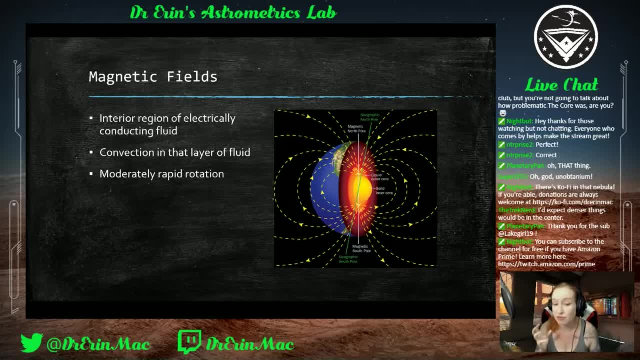 um electrically conducting fluid, a liquid part of your core. that's the main component, because you have to have a dynamic process happening in order to generate a magnetic field, And so if you don't have that, you're not going to get this magnetic field You need to have. 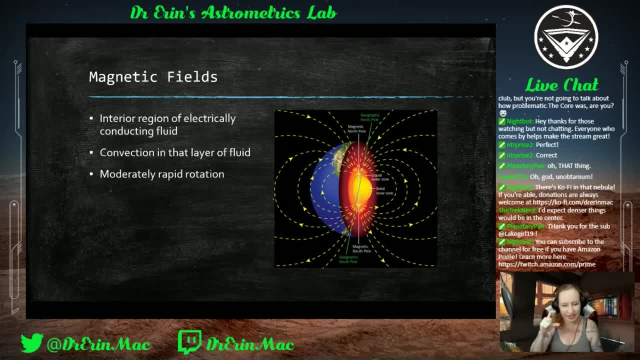 convection in that layer of fluid, So it can't all be one temperature. You have to have it hotter toward the center, cooler toward the top, such that you know to drive that process. So it has to be liquid So it can actually move. Then there has to be a temperature differential So it can 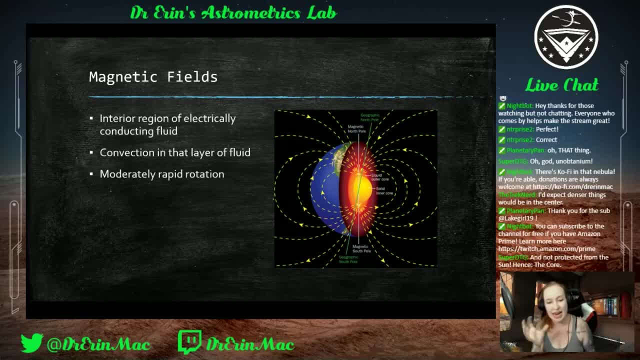 actually can, uh, go through a convection process And it has to be moderately rotating, which can also drive some of those dynamic changes. Um, and and not protected from this right. So, um, so, when you have this liquid outer core, 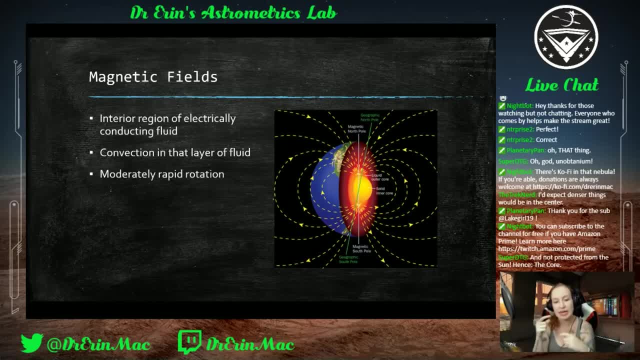 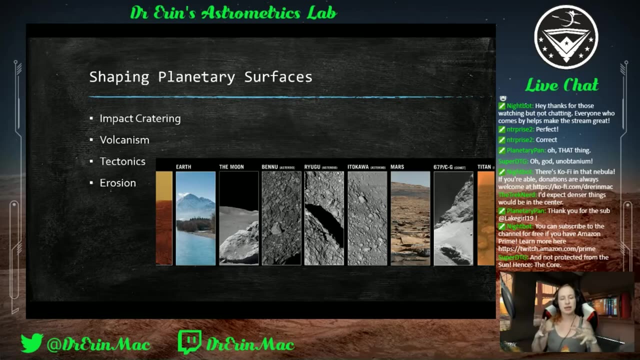 the fact that you have temperature differentials, the planet is rotating um and that it's liquid itself. all of that is what contributes to generating a magnetic field around or in the planet, Um. So. So that's how we get the center of planets and how we have some planets have magnetic fields, Some 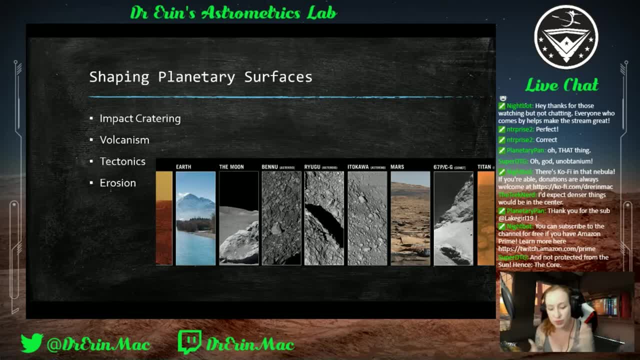 planets don't have magnetic fields. Now we'll get into each one individually. We'll talk about earth versus Mars. I know I've touched on Mars quite a few times here, but um, but it's really important once we get down to that specifically and we'll learn individually about each planet. 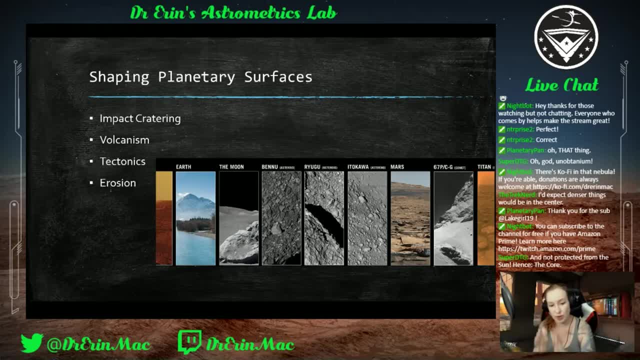 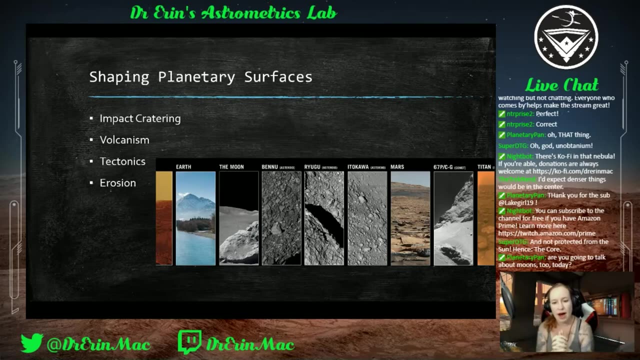 talking about why Mercury's core is the way it is, why Venus is the way it is, why more, uh, earth and Mars are. So that's how we get the center of planets and how we get the center of planets, Um. so let's move out. Now we've got how we got the core, how it heated up, how it's cooling off, Um, 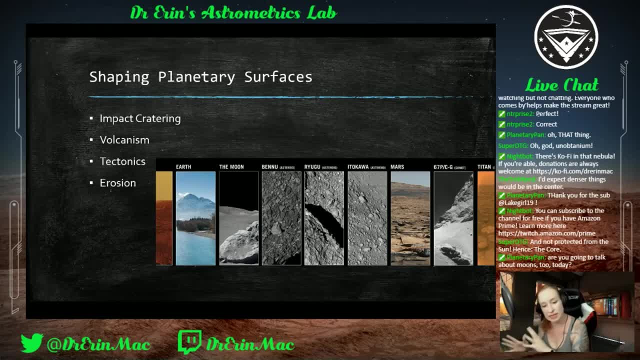 we'll talk a little bit about moons today. We're not going to be touching on the Jovian moons right now, Um, but yeah, not not today. We'll get into the specific bodies, uh, next week, Not sure if. 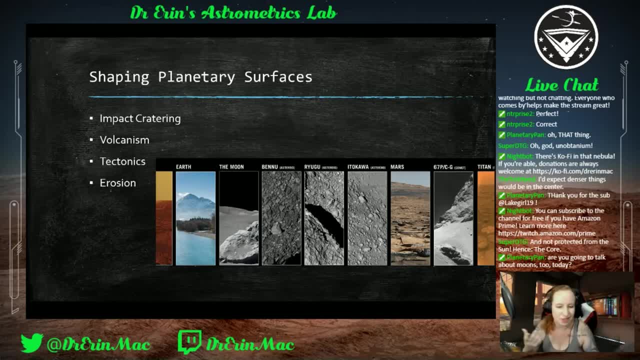 we'll fit in Europa next week, but that's just the one I'm most excited to talk about, Cause it's amazing, Um, but first we want to talk about, just in general, how these surfaces of these planetary bodies look the way that they do, And there's four main components that contribute to. 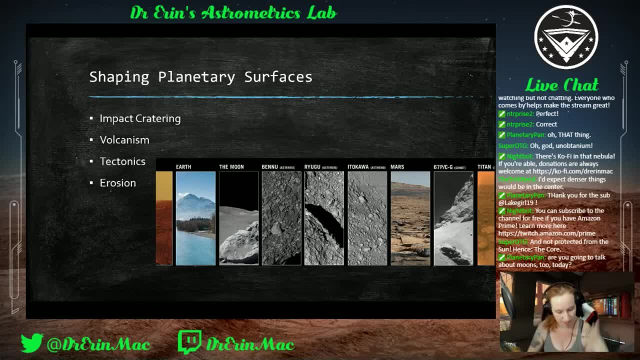 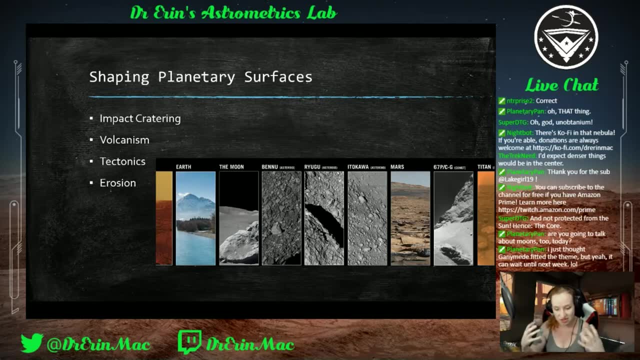 the surface of these, um, planetary surfaces. Uh, first is impact cratering. So this is the you know. stuff crashes into it. We get an asteroid impact. Um, oh, yeah, fair enough. Ganymede as well. Yeah, that's fair. Um, we also have volcanism. So volcanism is this eruption of. 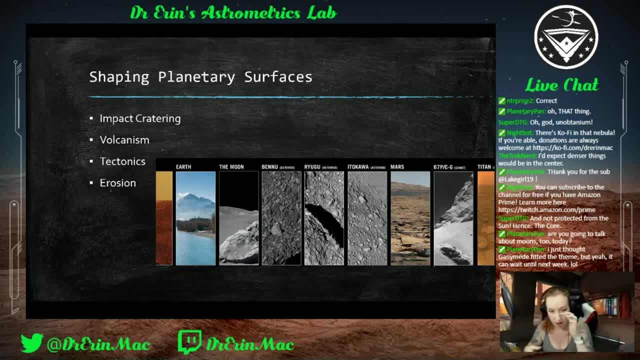 molten rock or lava from the interior onto the surface, Um, that kind of you know. it's again one of those things where we talk about volcanoes everyone's like, yeah, okay, I understand what a volcano is, but it's it's it's thinking about it from a definition standpoint and understanding. 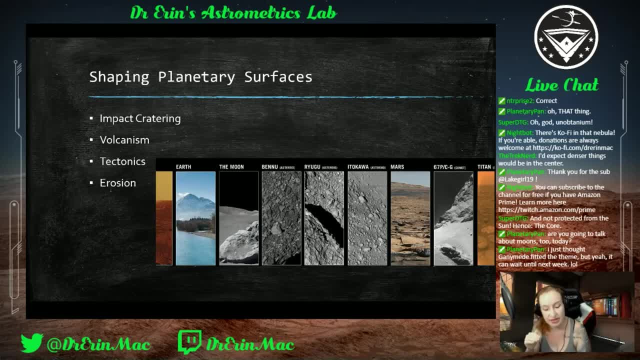 what processes are going on to that. So that's where we have this, this, you know, liquid material underneath the surface That is then being sent up to the top through a volcano. Then we have tectonics. So that's where. 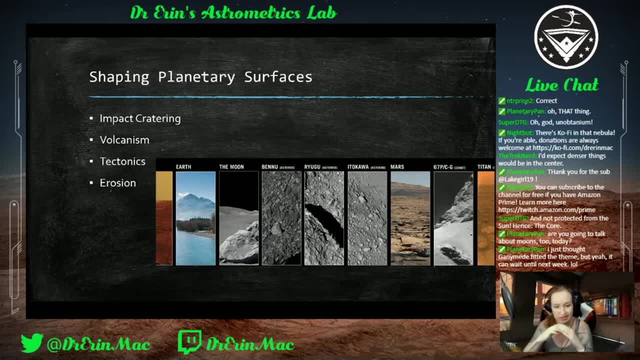 you have internal stresses on a planet, on the crust, um, are going to cause that crust to move and shift and go through tectonics, Um, and then erosion. So this could be things. this is a, you know, atmosphere, water, any of that stuff, It's just the wearing down or building up through wind. 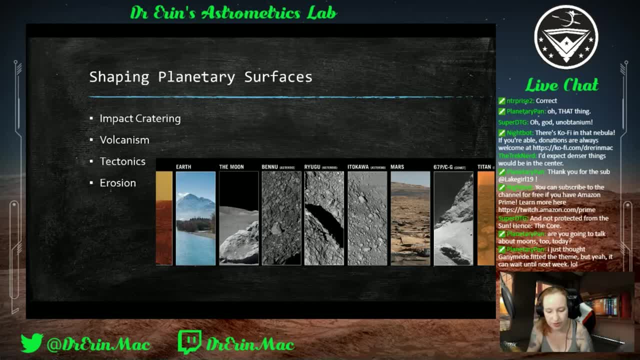 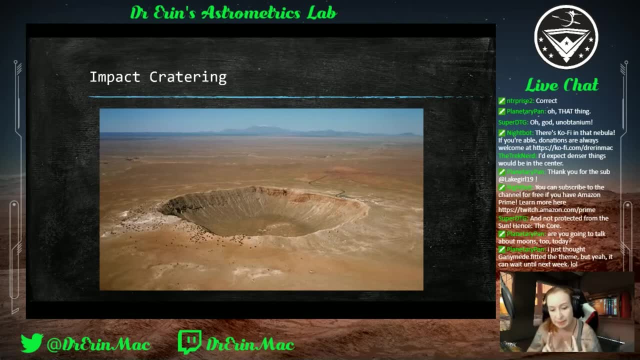 water, ice and any other sort of planetary Weather that that we have here. So let's talk about impact cratering. Now. this is primarily seen not necessarily on earth or Venus, though, as you can see here, it's not exclusive, um, because we 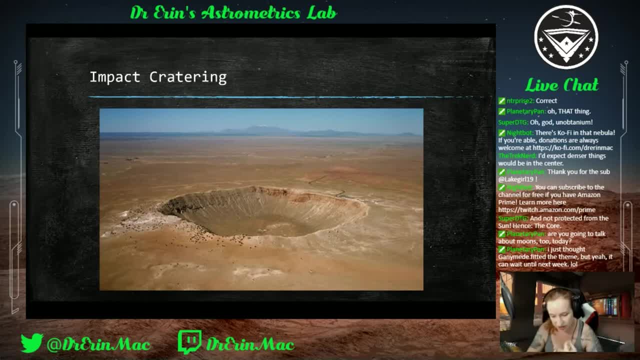 go through erosion. but impact cratering is very much seen on the moon and Mercury And that's just because they've they've taken beatings from comets, asteroids, all of this stuff, And because they don't have a um atmosphere, those don't go away. The other important thing about impact craters is that um 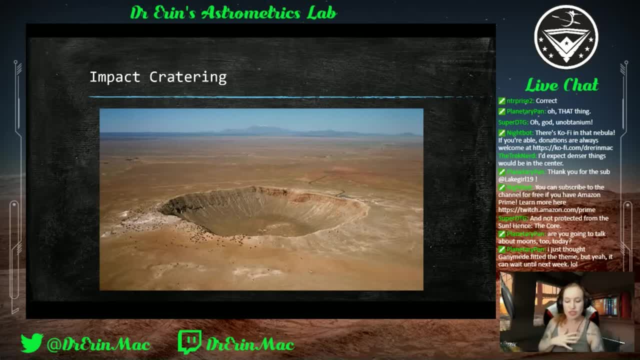 small craters outnumber the large ones, which helps us start to understand how many small objects versus big objects, what the distribution of objects is in our solar system, Because, remember, asteroids are actually really, really, really hard to see. They're incredibly dark, incredibly cold. 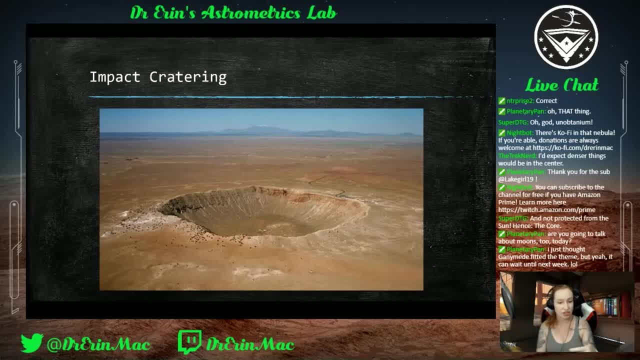 So they're not going to be giving off a lot of heat. They're not giving off radiation. They're dark, So they're not reflecting sunlight in the same way that, like ices are, So they're really hard to see. But if we can look at the impact craters on the moon or Mercury, where there's not an 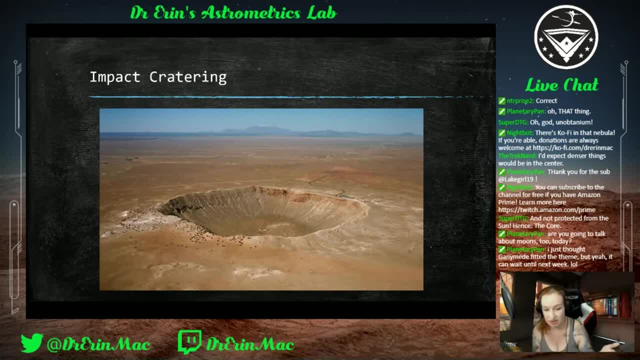 atmosphere, um, and as far as we can tell, there hasn't ever really been one. we can start to understand the history of our own, uh, our own, solar system here, Um, now, craters are usually circular, um, usually, because, uh, this impact blasts out everything in all directions. Um, you. 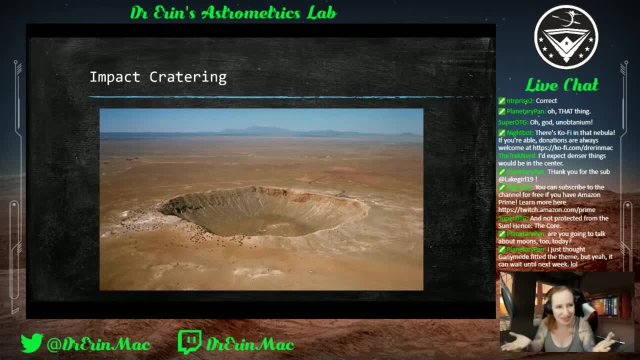 can do these tests. I mean it sounds kind of goofy because you see kids doing this at science museums, but it is legitimate research where you, you know, barrage a surface of you know maybe flour or something, and drop a marble into it and see how the distribution of material goes out. 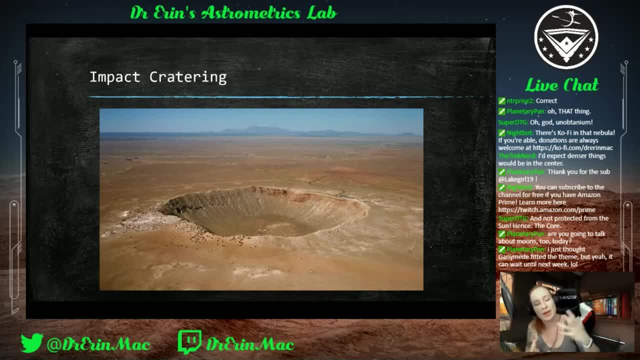 Um, so, understanding how many times you're going to get a circular impact crater versus maybe one that isn't circular, that is something that has been studied And we find that, um, that they're circular. Going through different other experiments, we can learn that 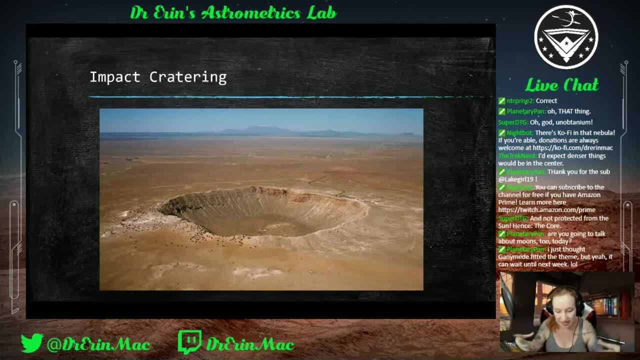 craters are typically about 10 times as wide as the objects that create them. So if you see one, divide it by 10 and you can estimate about how big the thing was that ran into it. Um, and about 10 to 20% deep as they are wide. So just if you can only look top down and you don't have the depth perception for you know, whatever reason, uh, you can estimate about 10 to 20% deeper than it is wide, And uh, so, for example, an asteroid about one kilometer in diameter will blast a crater about 10 kilometers wide. 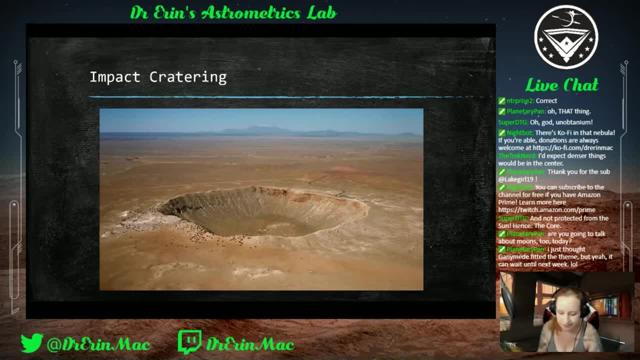 and about one to two kilometers deep. So those sort of um you know, tests you can do on this to try to figure that out. Oh, thanks, Vicar. Um, we also get uh clues about the geological conditions from impact craters and looking at crater shapes. Uh, so you can. 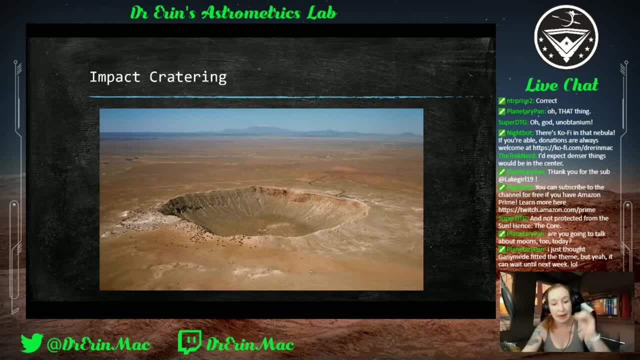 you can tell, for example, if you have like a bump in the in the uh bottom of it. So some of you have seen those. I'm sorry, I don't have a picture of them actually, Um, but if you have. 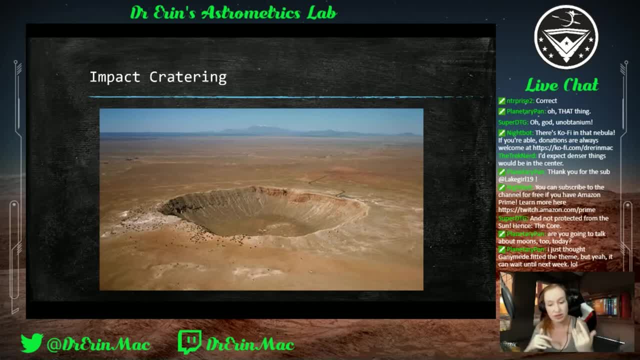 a bump in it that can indicate that, you know, maybe, that there is a little bit more viscosity, a little bit more, um, water, liquid ice, something like that, that could contribute to this bump popping up. Um, so, there's all these different things here. How much do atmospheres? 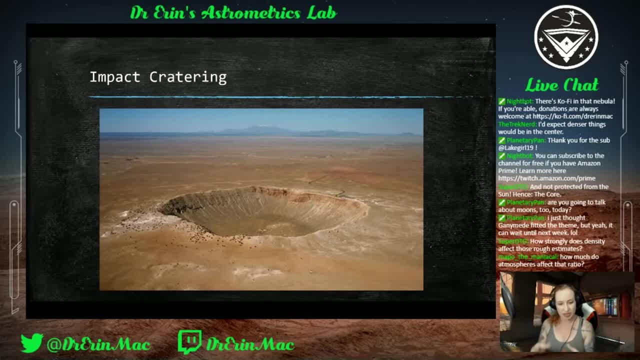 affect that ratio? That's a really good question. So that initial, initial, initial, initial initial impact crater, it's just going to be what specifically hit that. So that's not saying that essentially or effectively. let's say, for example, we take a five kilometer wide asteroid. 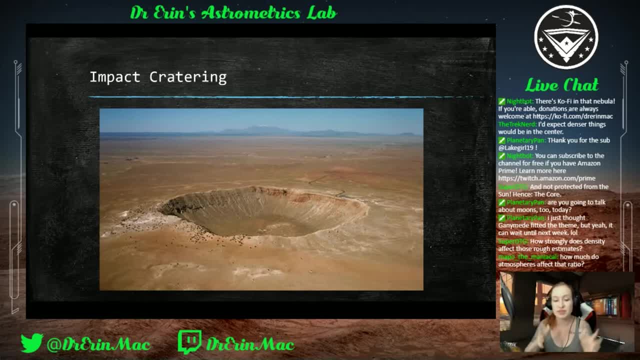 By the time it gets to the surface, if there's an atmosphere, it will have eroded away the size of that asteroid. So maybe it started at five. now it's only one kilometer. What we care about for the crater impact is just the size of it where it's going to hit the surface. So that's. 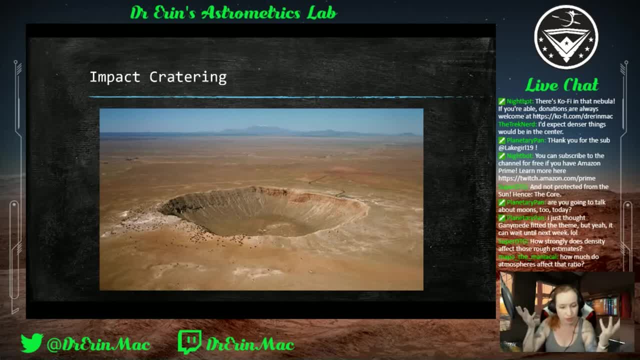 when it hits the ground. So it will lose matter. It will lose size by going through the atmosphere. So looking at impact craters on the surfaces of planets that have atmospheres are not necessarily going to tell us how big the asteroid was when it came through, just how big it was when it hit. 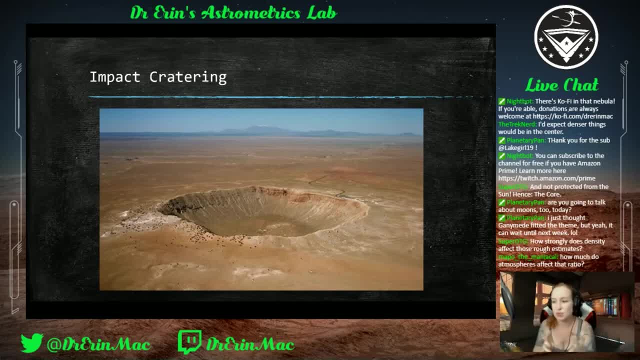 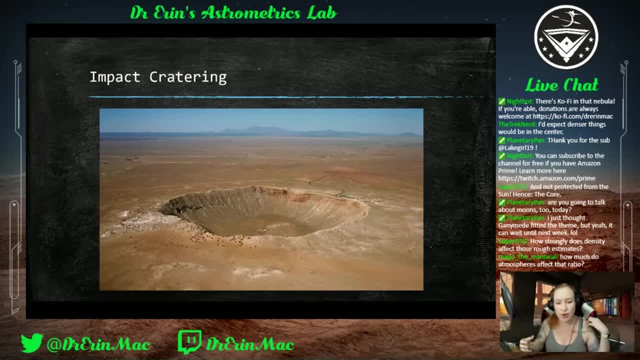 we understand our atmosphere, So we can say, okay, we saw. you know, the impact crater that killed the dinosaurs, for example. If that was X big and it went through our atmosphere, then it would have eroded this much. So that's how big it was before it came through the. 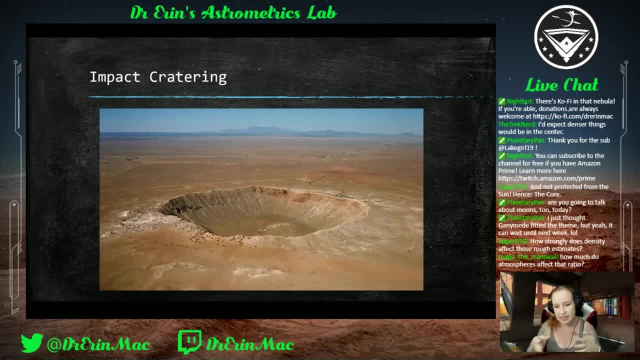 atmosphere. So yeah, the all of the sizes that I was talking about are just whatever object made it through the atmosphere to impact the surface. That's where that came from. And then Andy asked how strongly the density affects these rough estimates. Really good question. So because we get this differentiation with the material that forms. 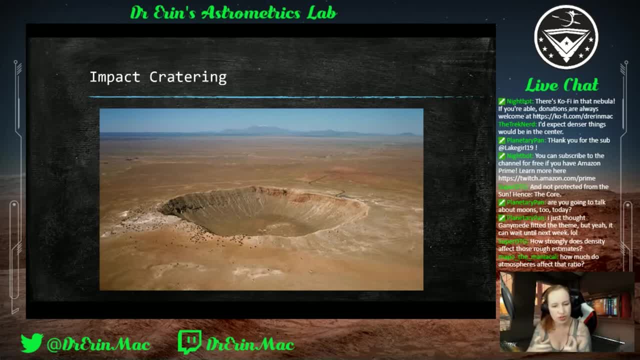 a planet. we have a good sense for that crust density because that's going to be the lightest rocky stuff that is present in our solar system, that made up the planets. So, for example, on the surface- and I again I have to check this up, Like granted. 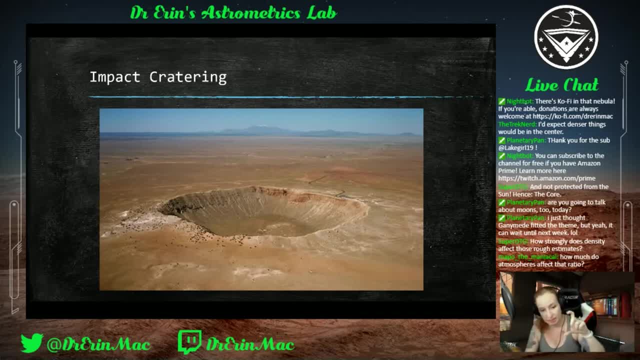 and basalt. Now, the amount of granite and basalt on the crust is going to be slightly different, but, for example, we're not going to necessarily get a metal crust on the surface. So when we're just talking about these rough estimates for impact craters, we're thinking light rocky material. 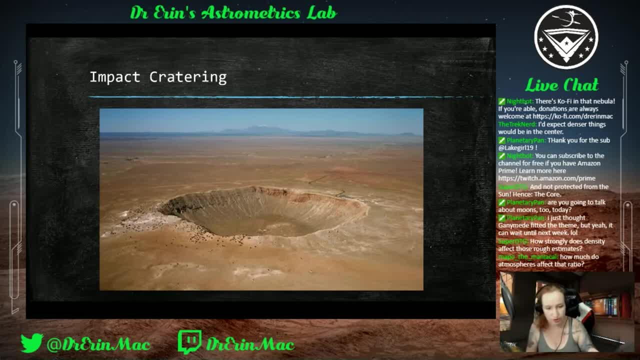 in general And in that sense those rough estimates hold up. Again, it's, it's about 10%, 10 to 20%. They're. they're rough, Rough, rough estimates, But for the most part because these very outer crusts are made up of a. 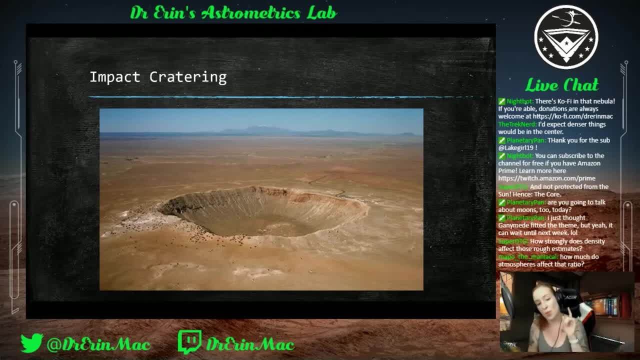 fairly similar material, it doesn't impact that much. What does impact- and that's kind of what I was trying to get to a little bit- is that the density affects the details of the shape of the impact crater. So, um, you have that typical bowl shape versus a bowl shape with. 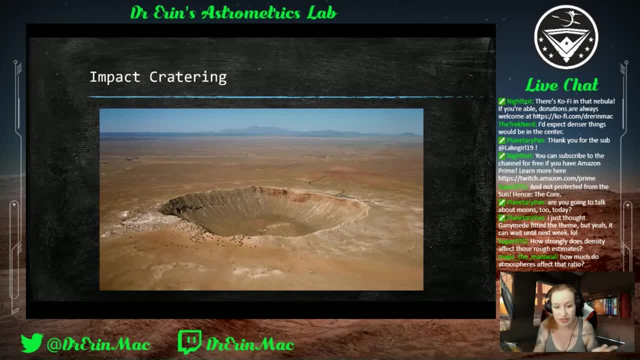 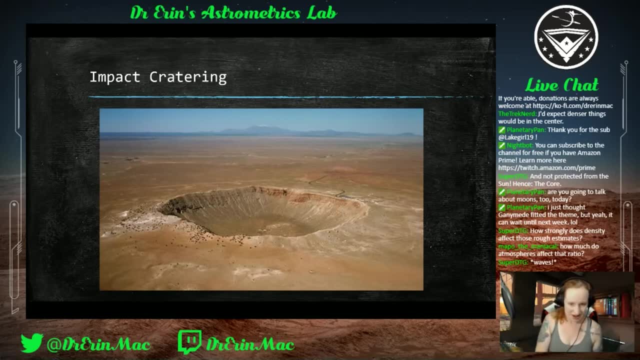 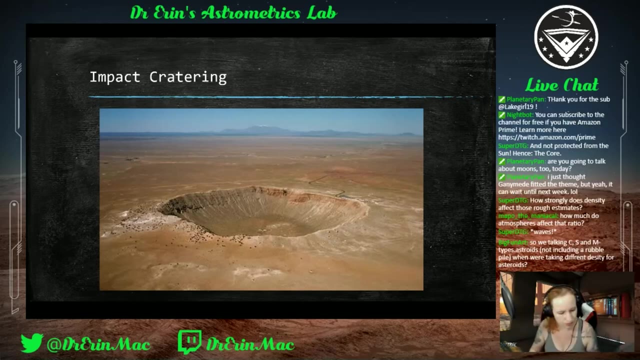 like a little bulge in the middle of it. That's going to more dictate the density of what it crashed into. if that makes sense, I hope that makes sense. Okay, cool, Awesome, All right, So, um, then we get, uh, volcanism. So let's go into that Volcanism, Um, 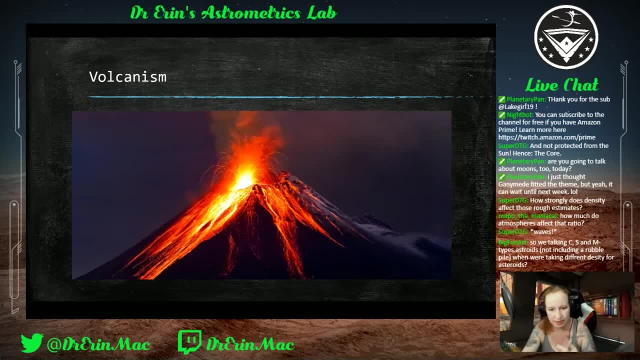 uh, so we're talking C, S and M type asteroids, not including a rubble pile. We're talking about different density for asteroids. Oh, that's a good question. So I was referring to the density of the asteroid itself, not the density of the asteroid itself. If that's what the question is, that's. 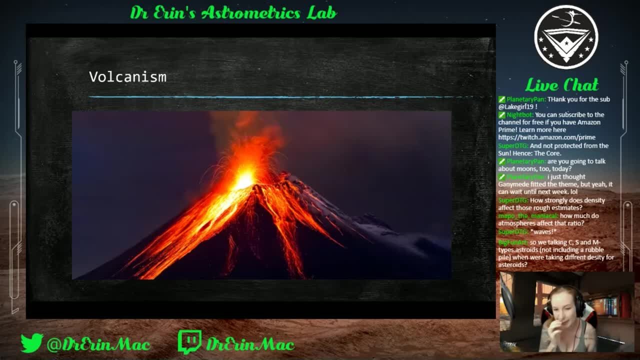 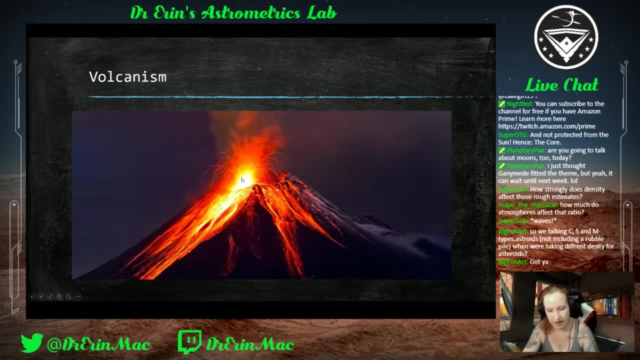 that's a little bit different. That's a good point, Um, but yeah, we can. let's look up those different because I don't know- I don't have those off the top of my head- what those are made out of. um, individually, How the density of the asteroid affects it. I think the density 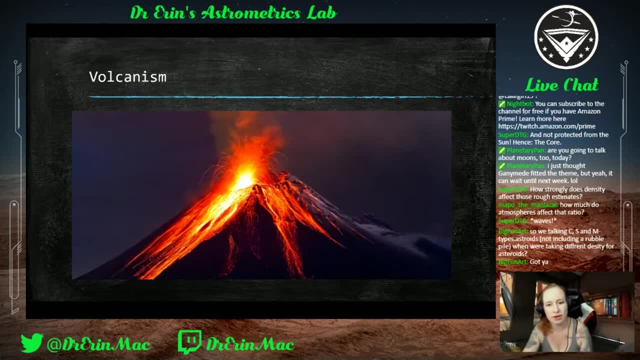 of the asteroid affects more how- ah, let's okay, let's think about that for a second. The density of the asteroid affects more how much it's going to erode in the atmosphere versus what type of impact crater it's going to make. And I say that because, if you're going to 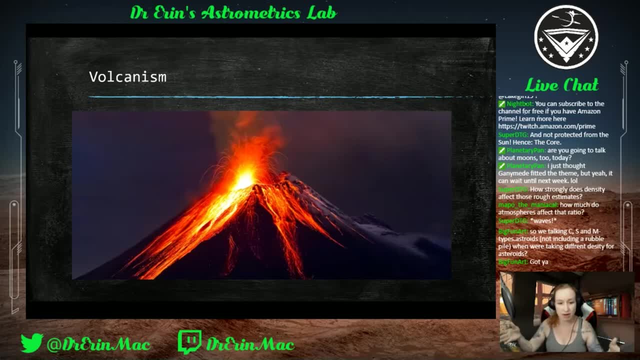 do a science experiment where we have a you know tub of flour and I drop a um, I drop a ball bearing versus a marble. they're still going to fall at the same rate. They are still going to make a circular impact crater. 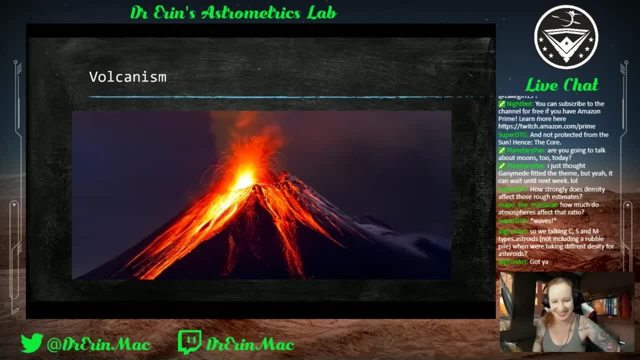 I really want to do a science experiment And I don't have a stop for it. But anyway, we'll, we'll. we'll dig into that a little bit more once we get through this. but thank you, That's a good question. All right, So volcanism. 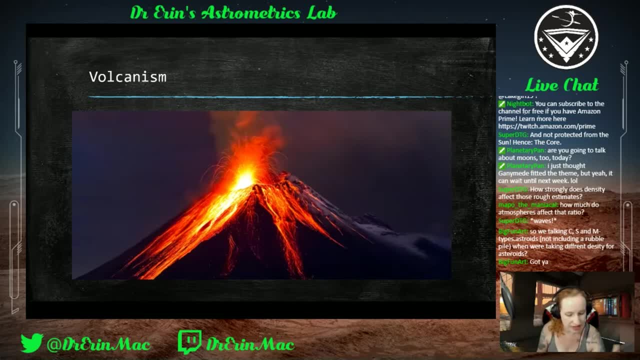 this is any type of molten lava, whether it's a you know tall volcano or it's just risen up through the cracks. um, it's just. volcanism occurs when you have an underground path, uh to magma makes its way up to the surface, Um, so molten rock tends to. 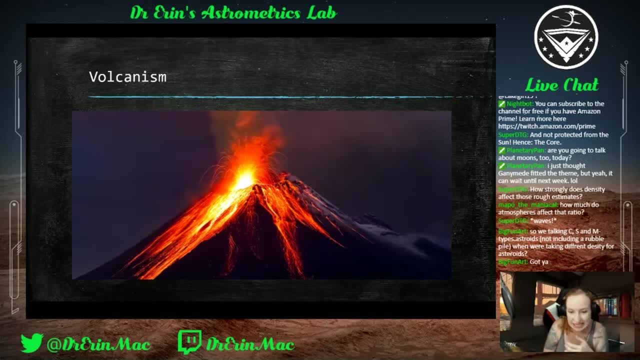 rise for three main reasons We have: molten rock is usually less dense than solid rock And, uh, so it's kind of differentiates itself because most of earth's interior is not molten. the solid rock surrounding a chamber of molten rock can squeeze that stuff, driving it upwards. 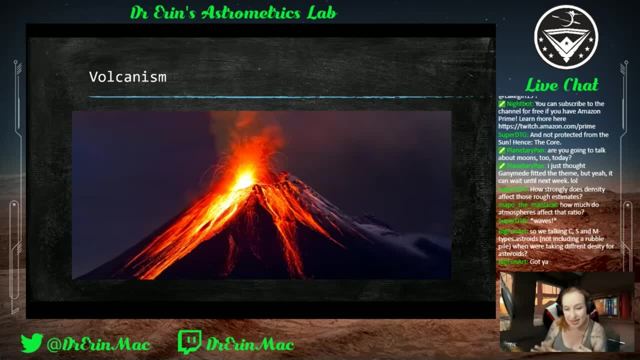 And then the third thing is: the molten rock often contains trapped gases which expand as it rises, because there's less pressure holding on. So as it rises, those bubbles expand, which is going to drive it further up as well. Um, and that's how you get these dramatic eruptions that comes. 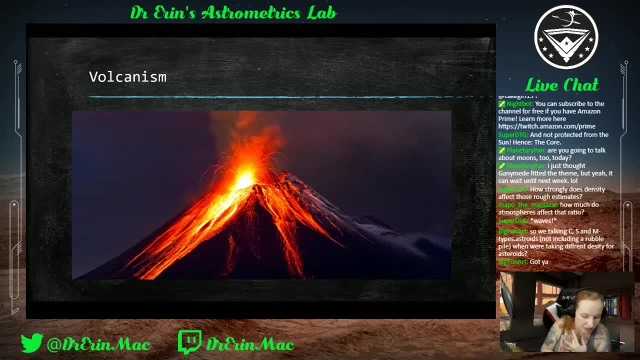 up. Uh, the results of these eruptions depends on how easily the lava flows on the surface. Um, so you know where you're thinking about. you know these examples: where it's really runny, really hot, it's going to flow a lot faster. versus thick lava, It's just more going to. 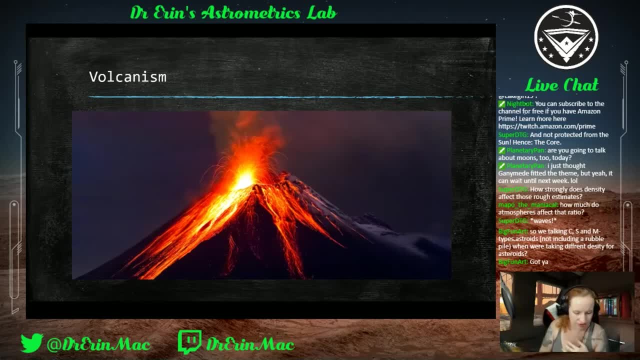 pool in one spot. Um, so these runniest lava flows, uh, the runniest lava flows really far and flattens out before solidifying. That's how you get those planes. and then, um, thicker lava solidified before they spread out. That's where you get those like shield volcanoes. 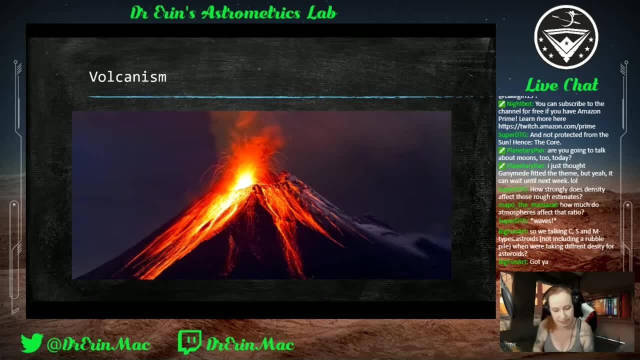 Um, which are can be very tall but not very steep. So things like, uh, the Hawaiian islands, for example, are these shield volcanoes, And then the thickest lavas can't flow very far before solidifying and build up tall, steep, what we call stratovolcanoes, And that's going to be like. 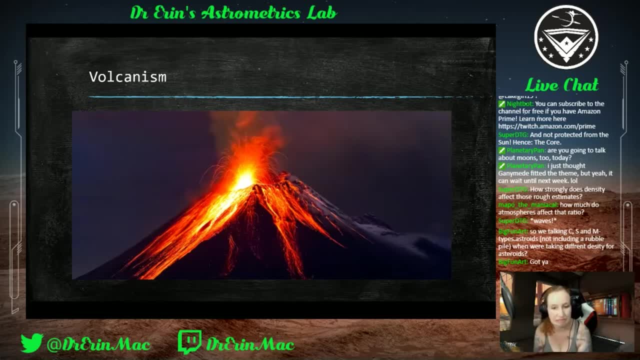 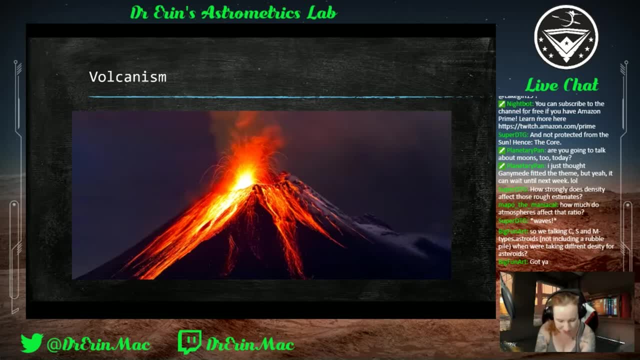 um are made out of and uh, yeah, let me see if there's any other details. Like I said, I mean this is astronomy 101.. It's not necessarily a geology course, so we don't have to get to all. 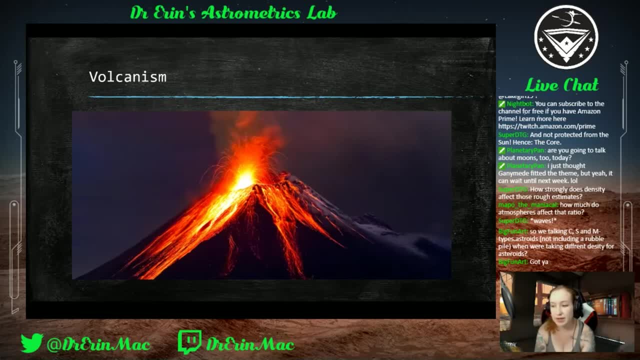 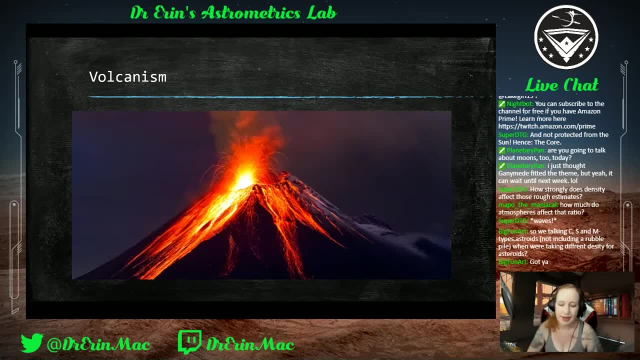 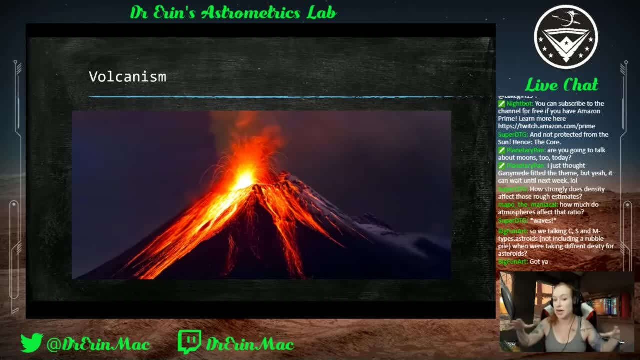 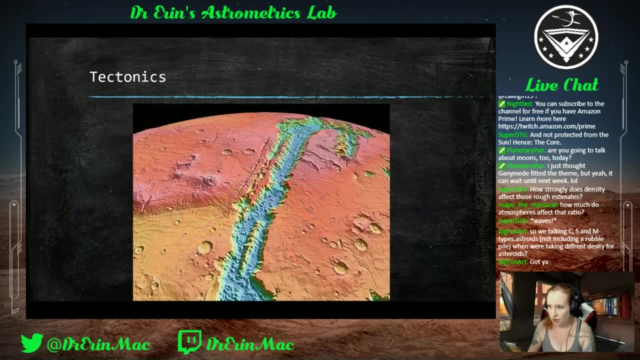 It's very so, it's very tall, but it's not steep, And um, and that's that tells us a lot. It tells us about the consistency of the lava that formed Olympus Mons, which is pretty cool, pretty interesting to think about, All right, And then we get tectonics. Um, so tectonics here. 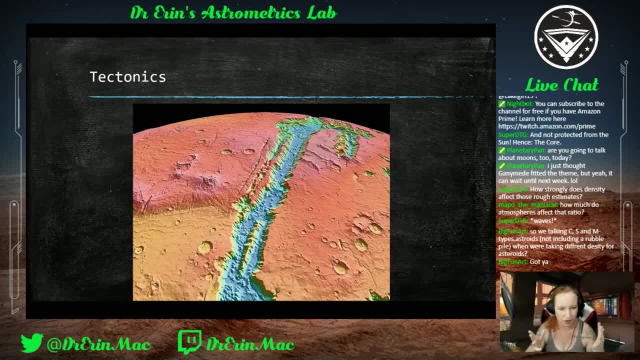 you know we talk about, uh, that particularly with Earth. I think we understand them pretty well- that how we get the different plates and how they move against each other, where you get that gosh. I'm not a geologist. 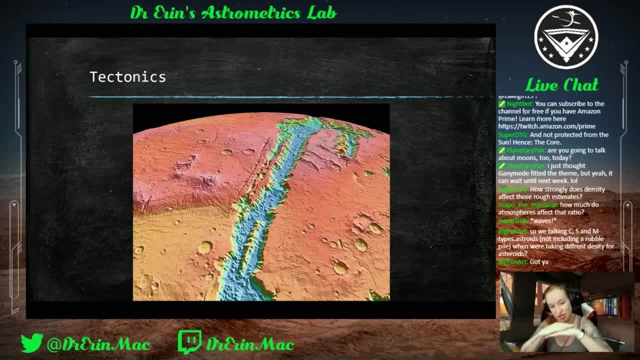 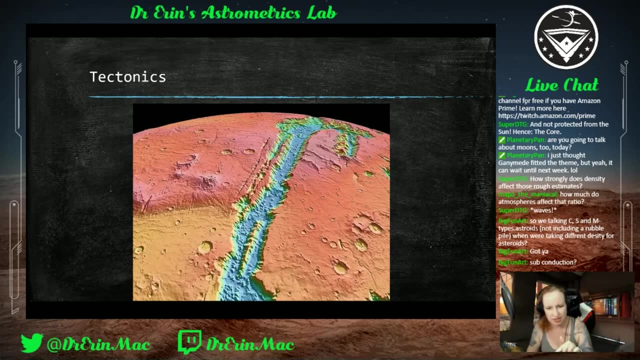 you can tell. You get the plates that go under the other plates, You get the plates that shift against each other, But all of those are being caused by these stressors that are inside of the planet's interior, And then these plate tectonics: subduction, subconduction, subduction. 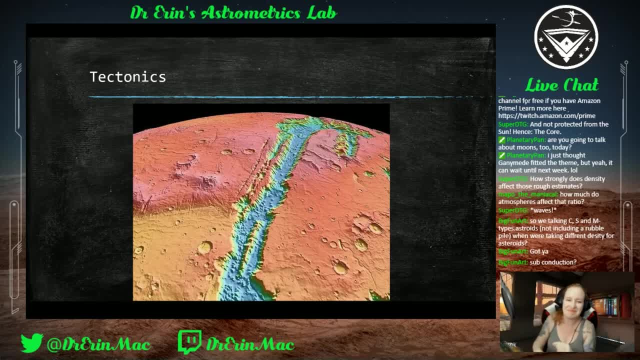 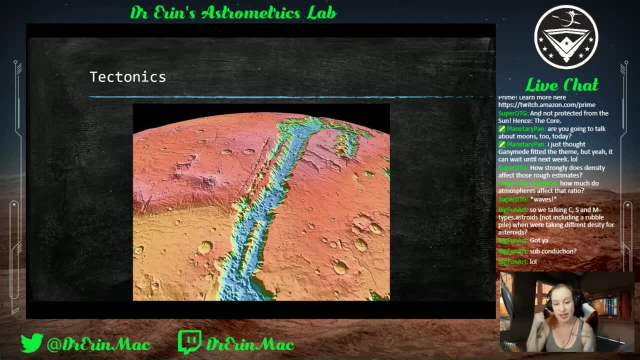 it's just subduction plates. I think We'll get there. I learned enough to know why I have earthquakes here in LA, and I learned enough to know why the Rocky Mountains formed in Colorado, where I grew up, And that's the only stuff that's stuck, But it still is important, though. 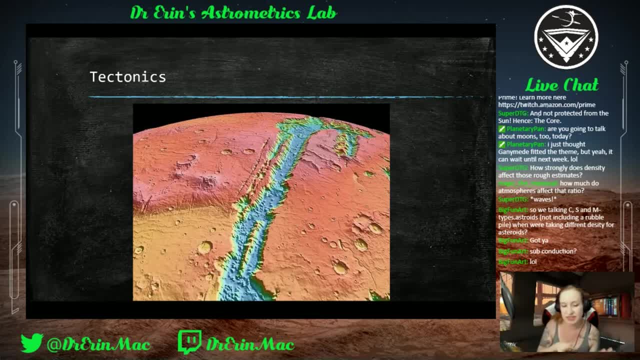 because if we're able to see tectonics or evidence of tectonics on other planets, that also can tell us a little bit about the history of the court, because it tells us how much stressors, how much pressure was put on the 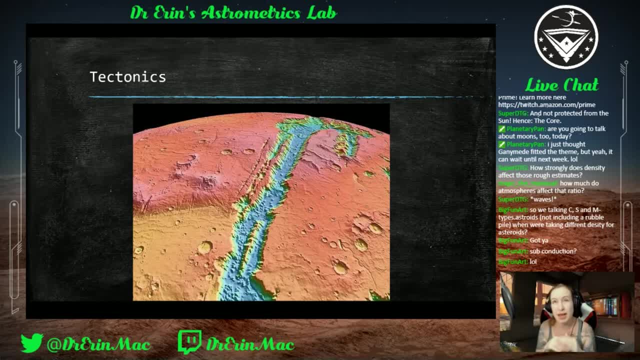 surface of the planet. If we have these plates, if we see past cracks, if we see mountain ranges that looked like they were formed, that tells us something about what the interior looked like, that it was liquid, that it did have stressors and different pain points that are on the surface. 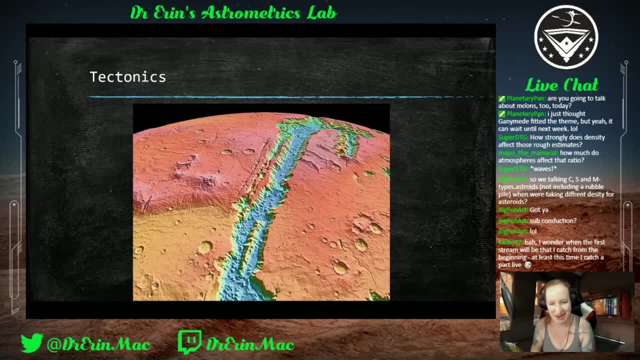 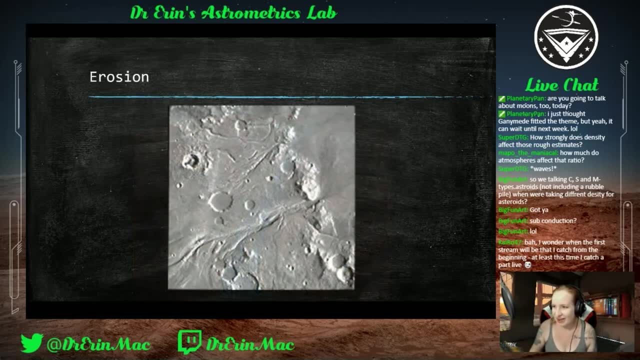 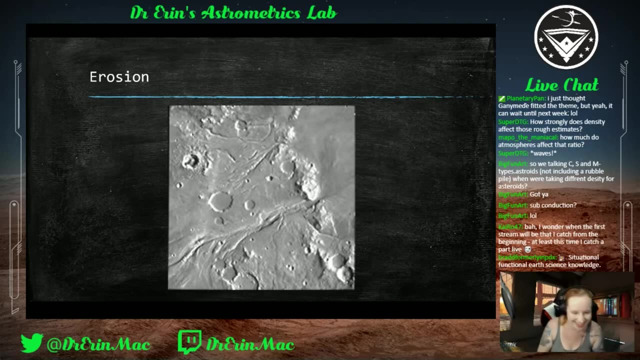 here. No worries, Cairo, Happy to have you here And, yeah, I'm glad you caught part of this live. No worries at all. All right, And then erosion. So erosion is kind of the to planetary geology, because it erases the history of the stuff that's. 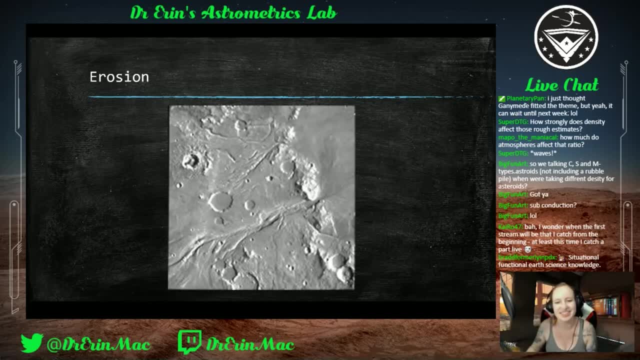 happened there. Thank you, Brad. Exactly, Situational, functional earth science knowledge. That's the extent of my geology. I know enough to be slightly dangerous, but only slightly, All right. So erosion is that breakdown or transport of surface rocks through. 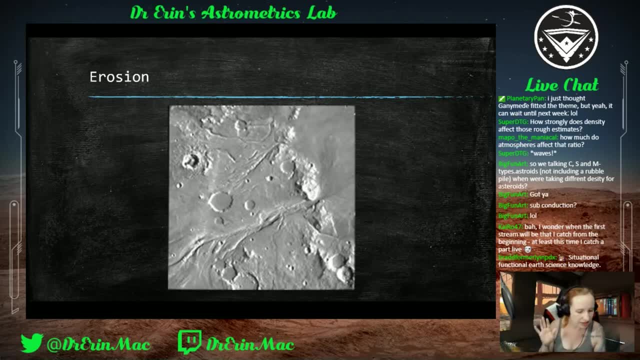 ice, liquid gas, So shaping valleys, shifting sand, all of those, And then, as Becca pointed out, this is also how we get sedimentary rock, that it deposits layers as we go- Really cool, interesting stuff. And you know it's important when it comes to also understanding. 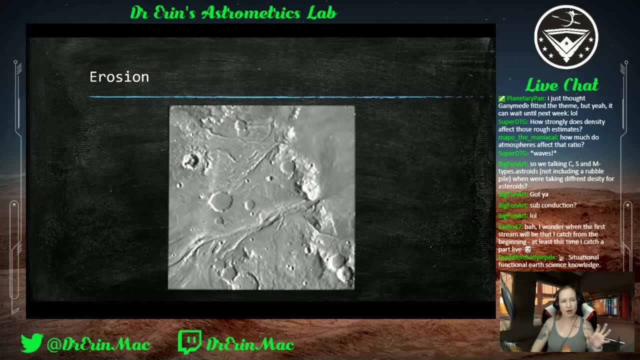 the history, even though it's a little bit annoying when we're talking about it. you know, Mars may have had- there's evidence that Mars had an atmosphere at one point, So that means that it did undergo erosion. So when we're seeing the surface, we're not seeing it as it was. 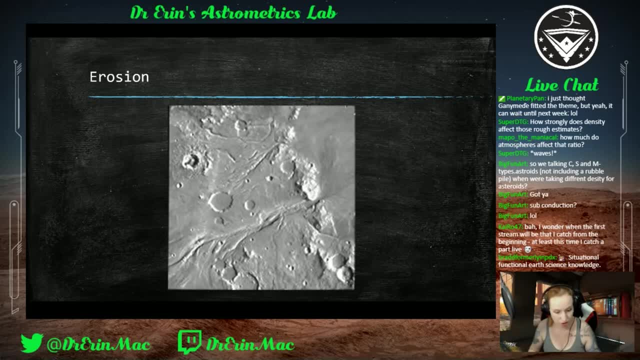 when it first formed, as opposed to when we're looking at Mercury or the moon. However, seeing what erosion we can identify on Mars also tells us something about its past. For example, we have the big crack Mariner Valley on Mars. We can look at that and understanding our processes of erosion. 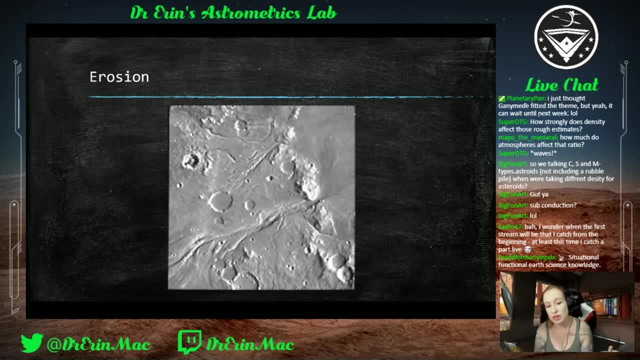 here on Earth that formed things like the Grand Canyon. we can look at Mariner Valley and determine that erosion did not cause that valley in the same way that the Grand Canyon formed here. So it can be used for good and for evil, to learn things and to rule out things. So it's still an important